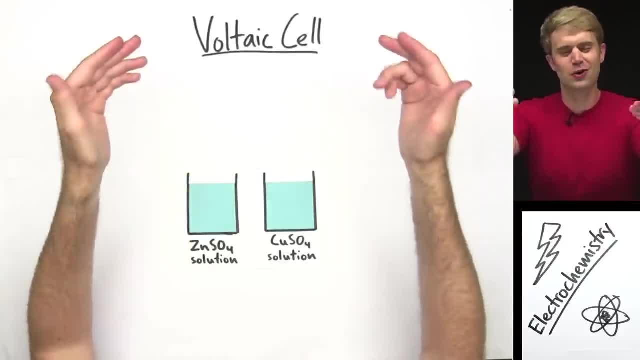 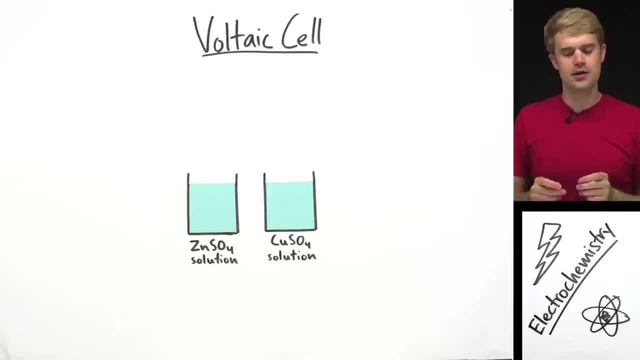 Okay, so I think for the rest of this video, I'm just going to call these voltaic cells, instead of calling them galvanic or voltaic cells. All right, so I now want to talk about the parts of a basic voltaic cell, One that that you could actually. 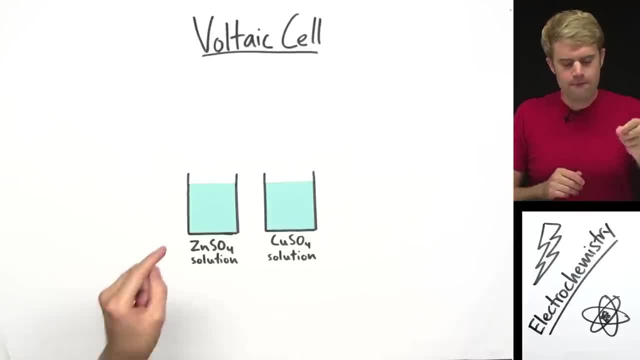 make in the lab. So here's what they are. First we start with two beakers or containers of water and into one of them we dissolve some zinc sulfate to make a solution, and then into the other we dissolve some copper sulfate and make a solution with that. So we've got these two solutions. 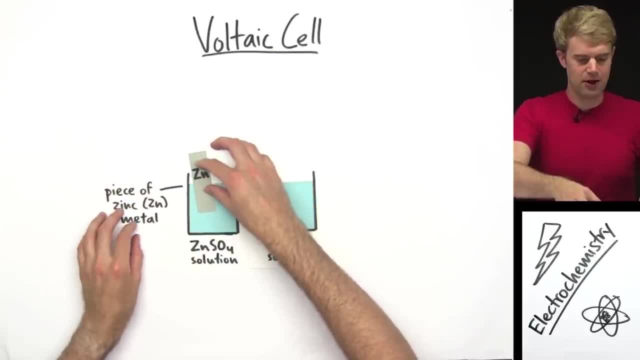 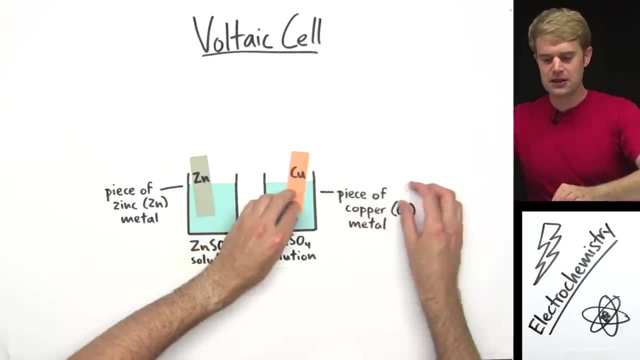 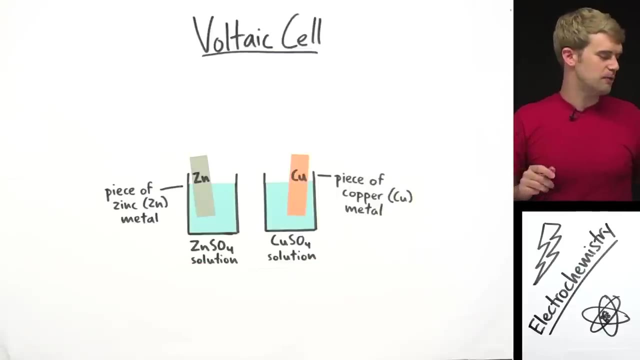 Then we take a piece of zinc metal, like this one right here, and put that in the zinc sulfate solution. we take a piece of copper metal and we put that in the copper sulfate solution. The next thing we do is we take a wire, a metal wire, and we use that to connect. 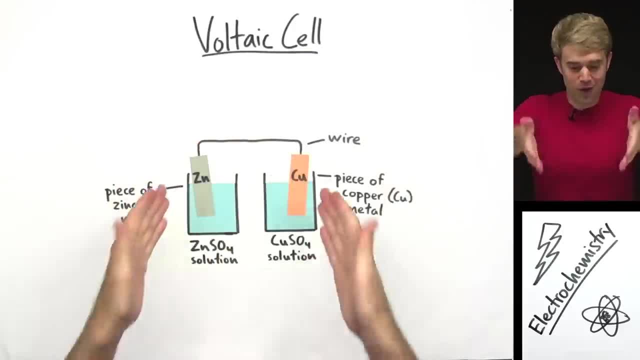 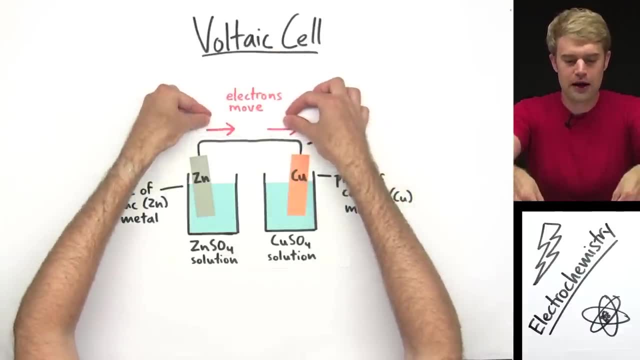 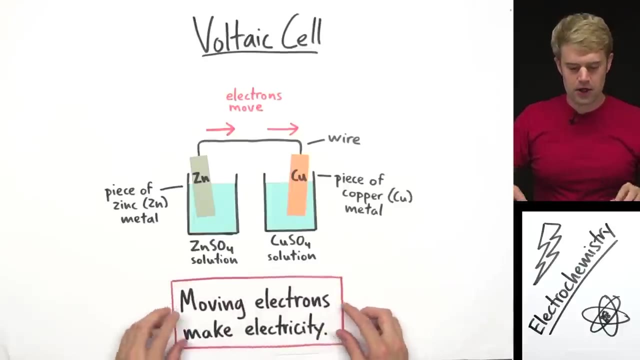 the two pieces of metal together. and when we do this, something amazing starts happening. Electrons start moving through this wire. They move from the zinc metal into the copper metal. Now, this is a big deal, because moving electrons are what make electricity. So when we hook this, 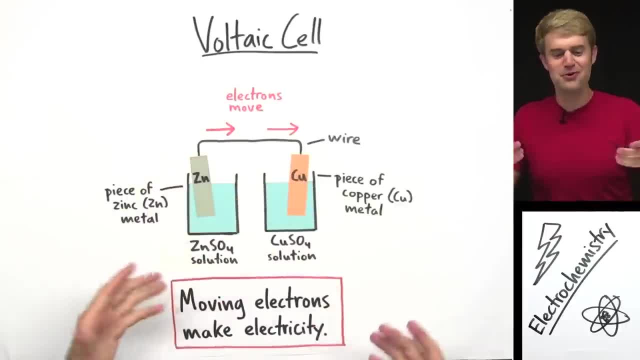 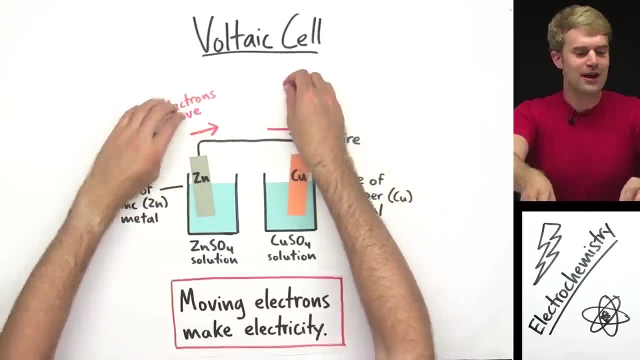 wire, together with the pieces of metal and electrons, start moving through it. we have electricity. We have electricity moving through this wire and what we could actually do is we could take a little light bulb like this and hook it up to this wire and the light bulb 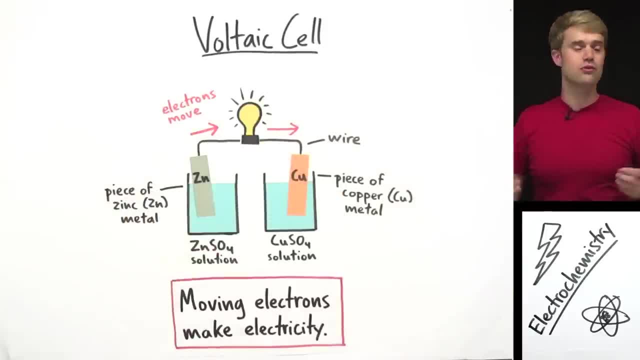 would turn on, because there's electricity moving through this wire. Now, to be really specific, there's one more part of the voltaic cell and that's a little tube called a salt bridge that connects these two solutions. We'll talk more about the salt bridge. 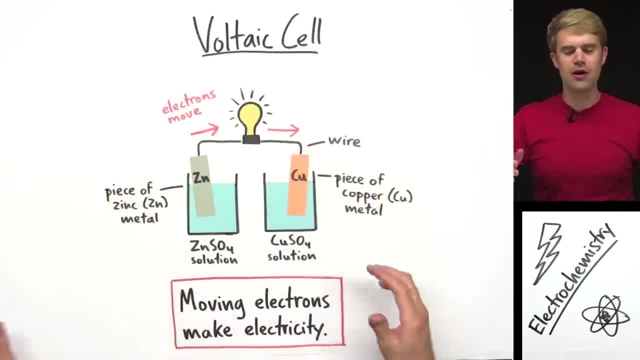 at the very end of this video, but right now I'm going to leave it out because I want to make sure that we keep things simple. So this is the basic setup of a voltaic cell. Now I want to zoom in the atoms and electrons in the metal and in the solution and understand what's causing. 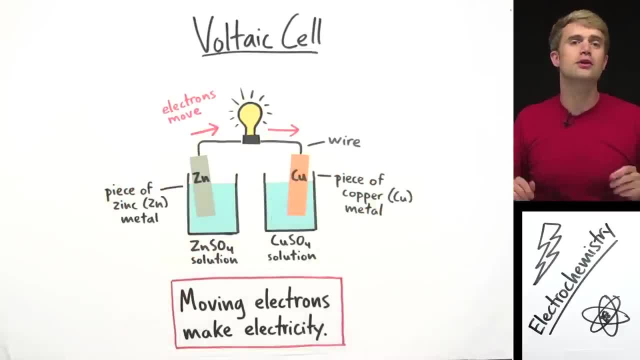 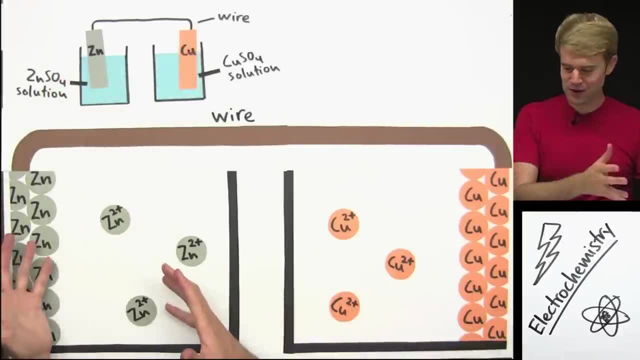 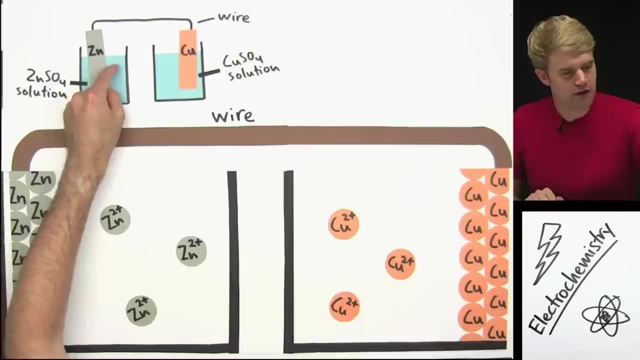 electrons to move along this wire and create electricity. Here's our magnification of the different parts of the voltaic cell. We can see some of the atoms in the metals and in the solutions. So let me show you what's what. This is a magnification of the area here. 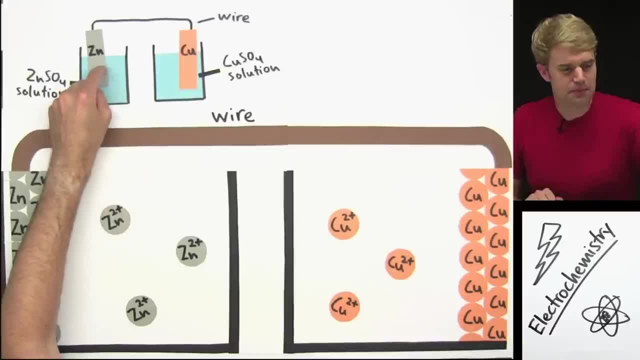 These zinc atoms are on the edge of the piece of the zinc metal, And then these Zn2 plus ions are in the solution. They're part of this ZnSO4 solution. I'm not showing the SO4 here, I just want to focus in on the zinc. 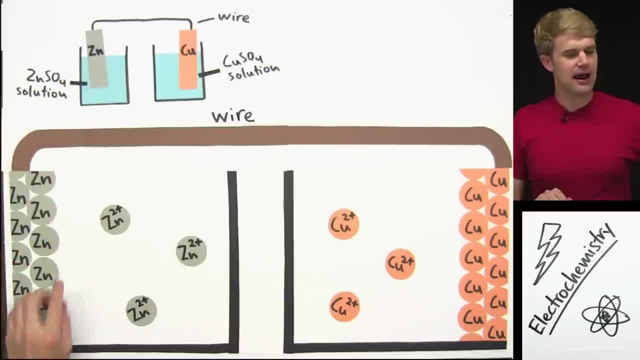 So zinc ions in the solution and these zinc atoms in the piece of zinc. Then over here we have these Cu2 plus ions That are in the CuSO4 solution. They're dissolved here, And then these copper atoms are on the edge of this piece of copper here. 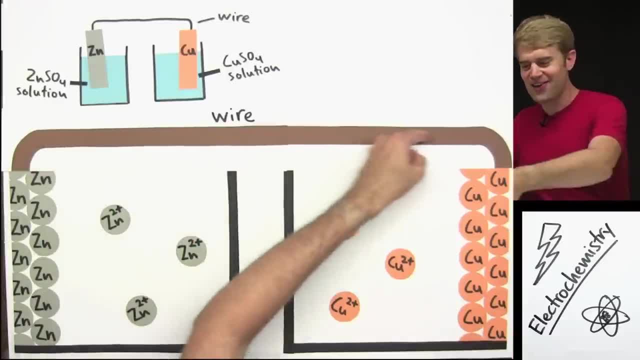 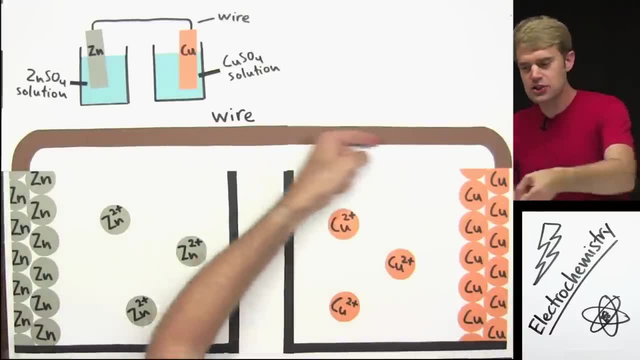 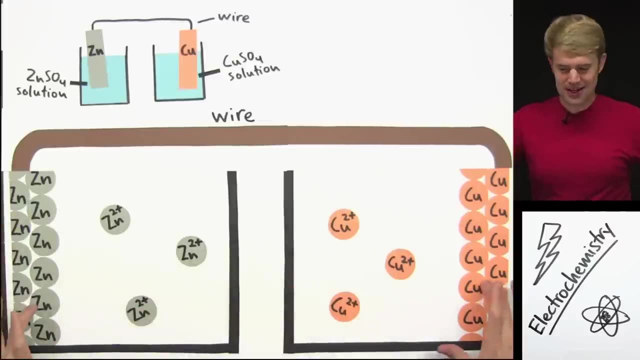 Okay, So we've got a wire that connects the zinc and the copper, And we've said that when we hook everything together, electrons start flowing through this wire. Well, why is that? Well, Because when we connect these two pieces of metal with wire, it kind of starts a tug of 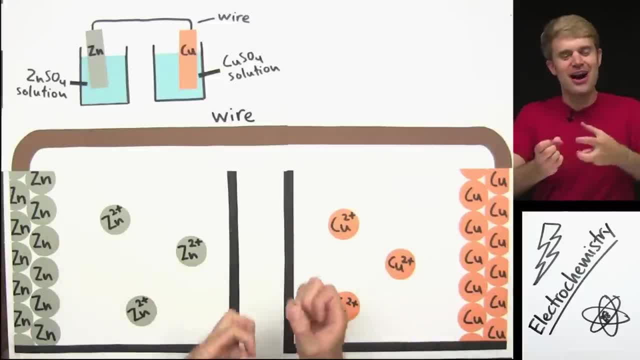 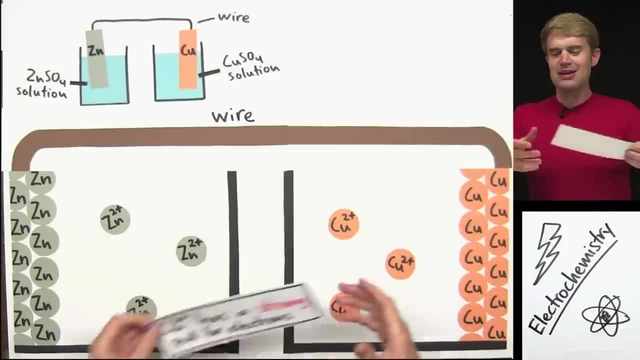 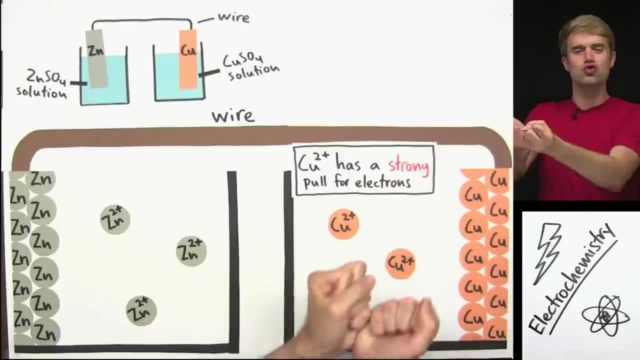 war between the zinc and the copper. They're having a tug of war for the electrons. One of them wins and one of them loses. It turns out that Cu2 plus these atoms here, Cu2 plus has a really strong pull for the. 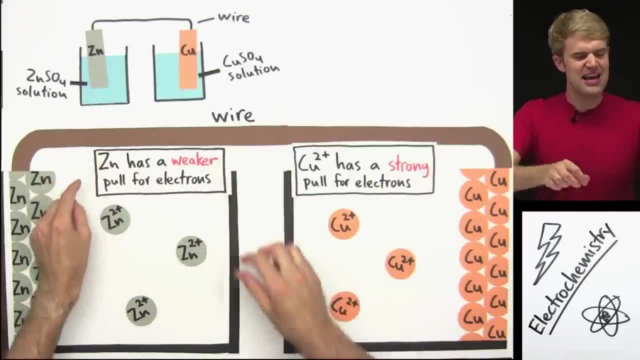 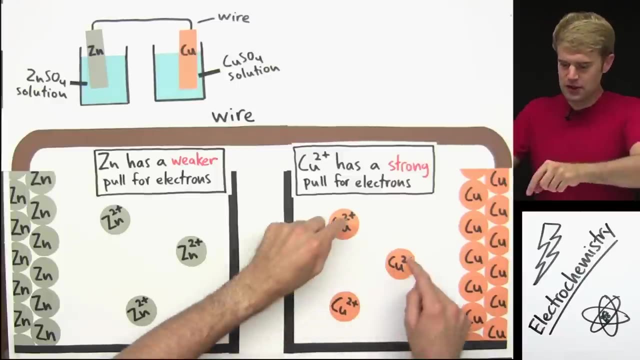 electrons, But then on the other hand, zinc, These zinc atoms. Zinc has a weaker pull for electrons. So in this tug of war, Cu2 plus ends up winning. Let me show you how this happens. So Cu2 plus really wants electrons. 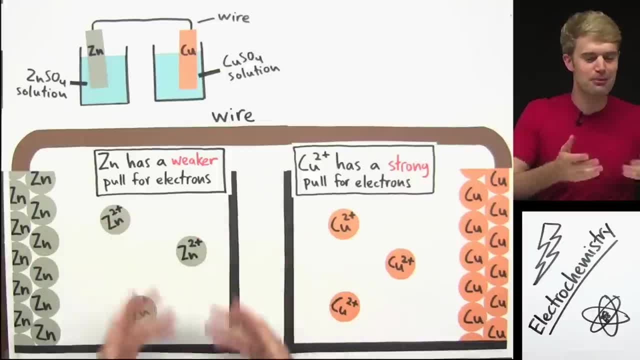 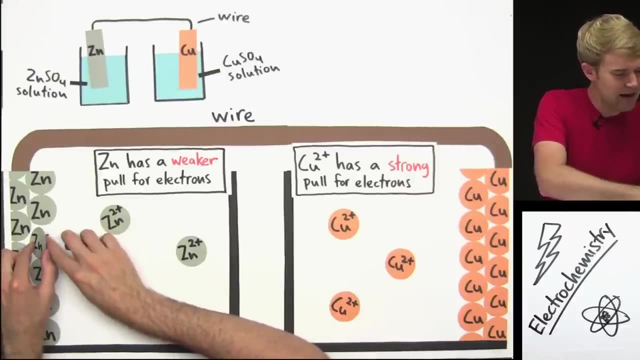 So it's kind of like it calls over here to zinc, which has a weaker pull on the electrons, and says, hey, zinc, give me some of your electrons And zinc's kind of weak. So it's like, oh, okay, Okay, And what happens is, let's say, this zinc atom here gives away two of its electrons. 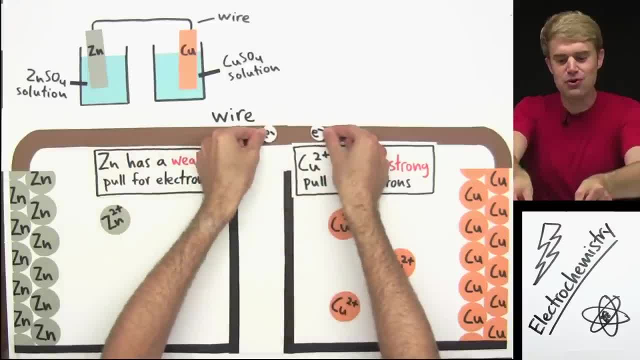 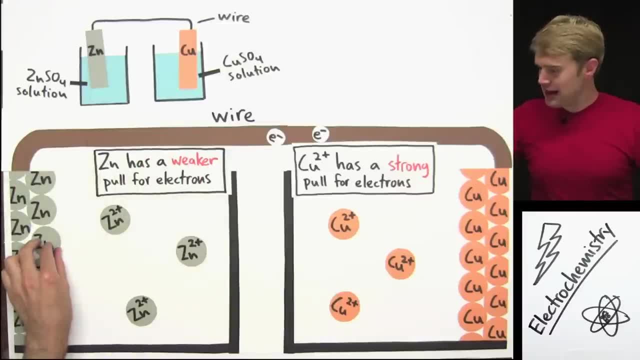 And these electrons enter the wire and move towards the copper. Now, when zinc gives away those two electrons, it causes its charge to change. It's lost two electrons, so it gets a positive charge and it becomes Zn2 plus. Okay, Now changing from neutral zinc to Zn2 plus has a big effect on this atom. 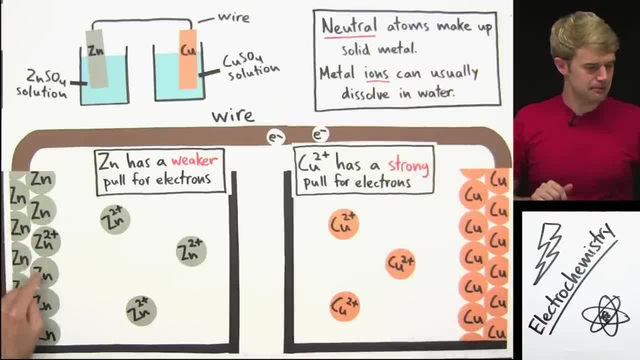 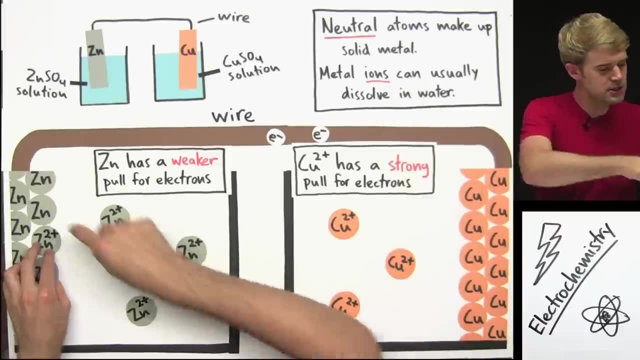 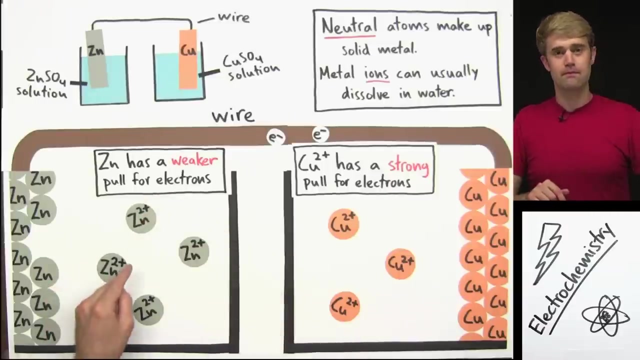 And that's because neutral atoms make up solid metal, but metal ions usually dissolve in water. So after this zinc atom turns into Zn2 plus, because it lost these electrons, it's no longer part of this solid metal anymore, Okay. And when it floats off, it dissolves into the solution. 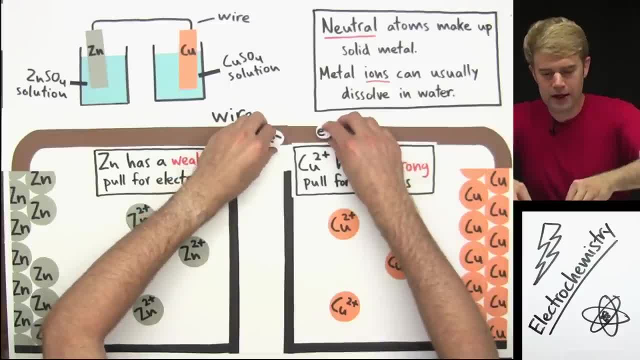 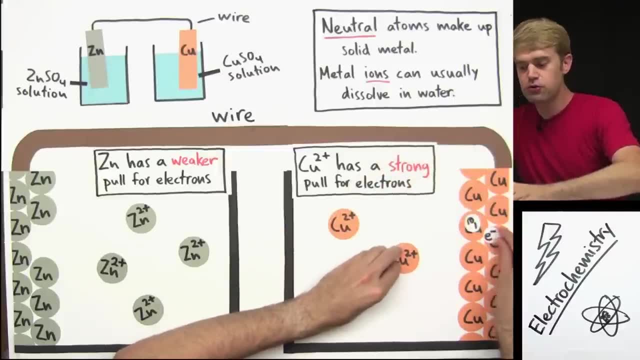 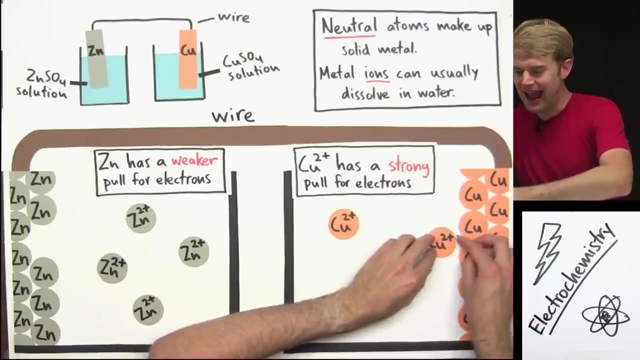 Okay, so that's what happens to the zinc. Then, over here, these electrons make their way down the wire to the copper and one of these Cu2 plus ions, which really wants electrons, is going to come over here and these two electrons are going to be added to the Cu2 plus ion. 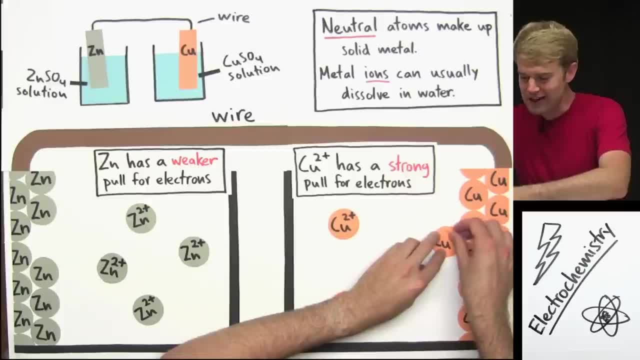 Gaining these two electrons is going to get really bad. So what happens is that the electrons are going to be added to the copper and one of these Cu2 plus ions is going to get really bad. So what happens is that the electrons are going to get rid of that Cu2 plus charge. that 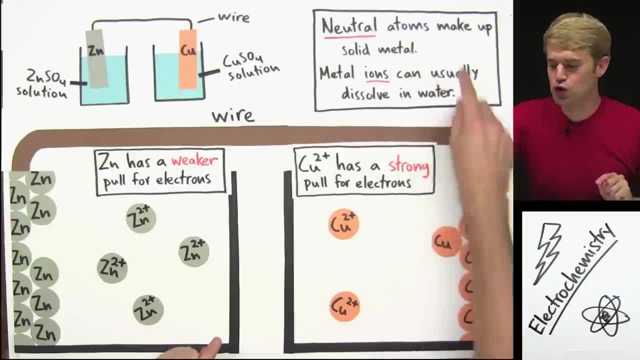 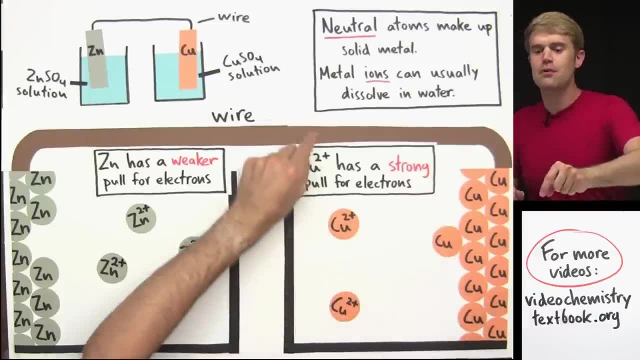 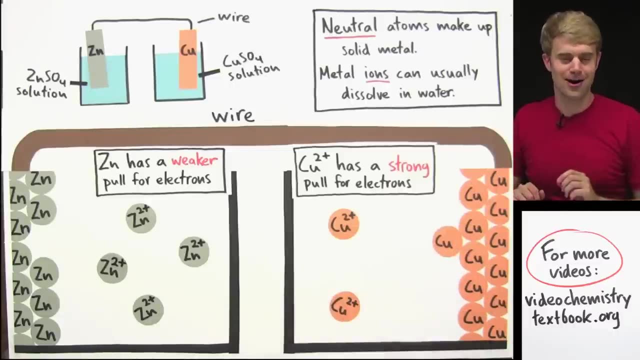 was on the copper and that is going to turn it into a neutral atom, which means that it is no longer going to be able to dissolve in solution and it's going to become part of the solid copper metal here. Okay, so that's what happens to the copper. 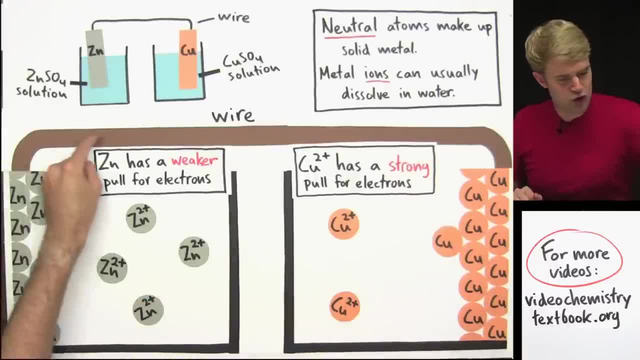 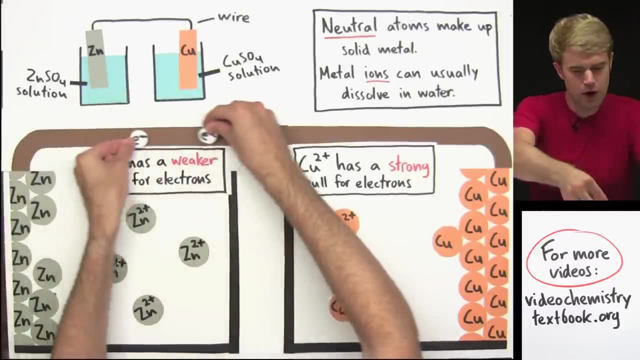 Now notice that for this whole process to happen, electrons have to move through this wire, And that's where the electricity, the electron movement, comes from. Let's see that one more time. So zinc loses two of its electrons here. Those move through the wire. 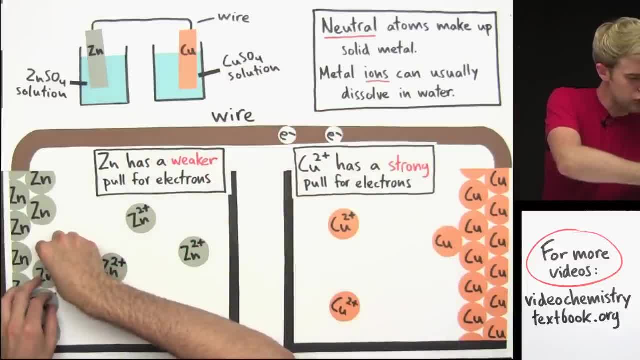 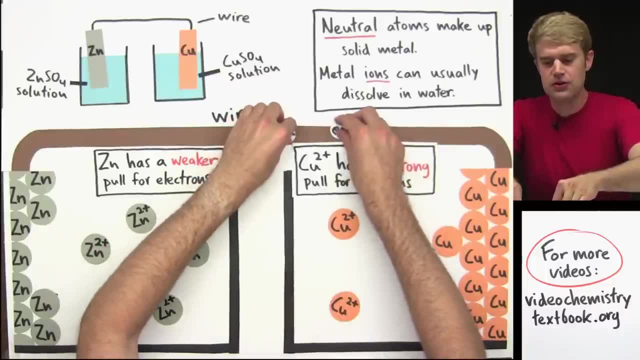 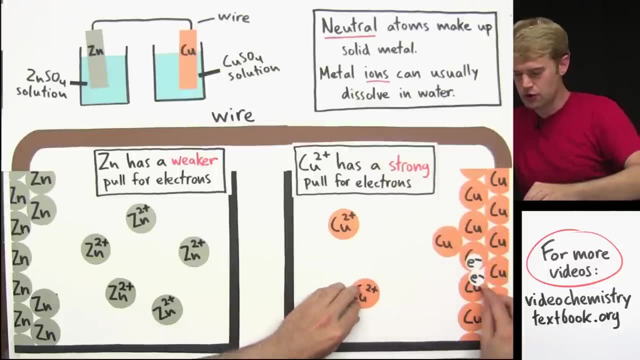 Loss of those two electrons causes zinc to take on a Cu2 plus charge. It is then going to dissolve in the solution. These two electrons are going to move over here to copper, And one of these Cu2 plus ions that really wants electrons is going to come. 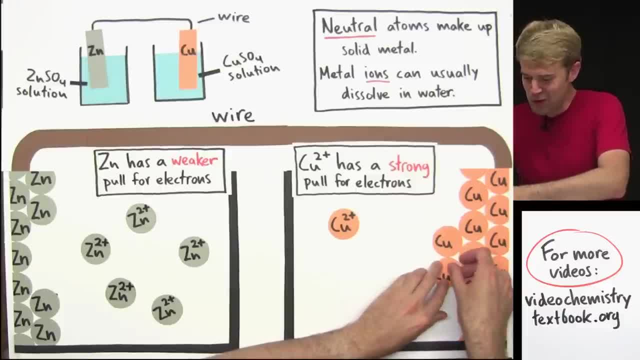 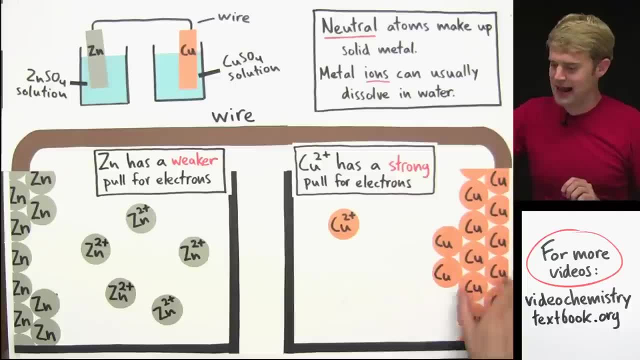 It's going to take them in and that is going to get rid of the Cu2 plus. It's going to get rid of the 2 plus charge and this neutral copper atom is now going to become part of this solid piece of copper metal. 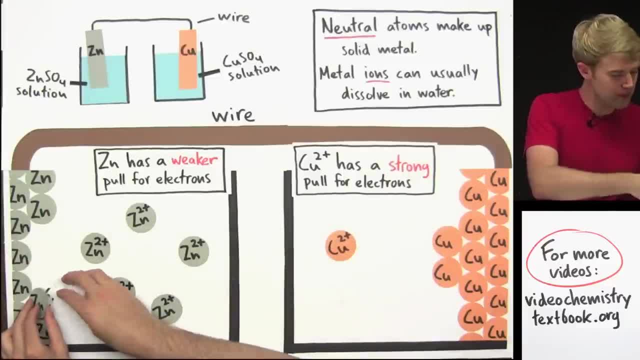 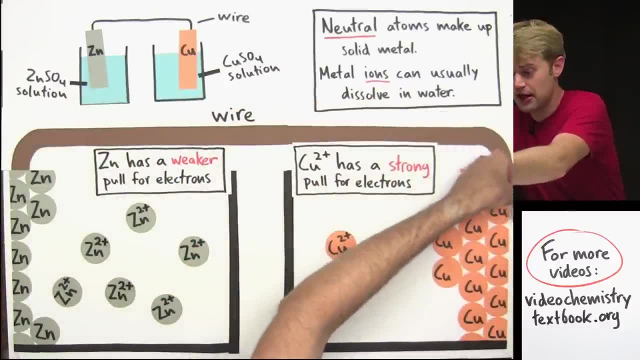 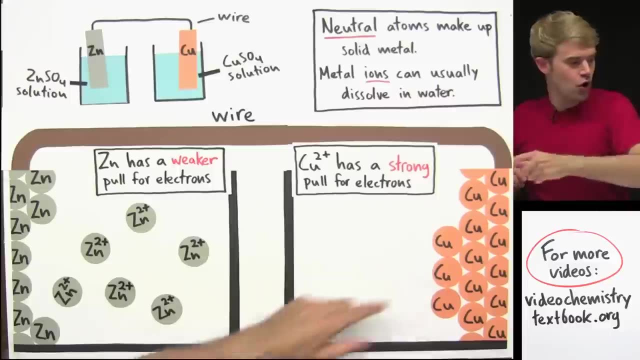 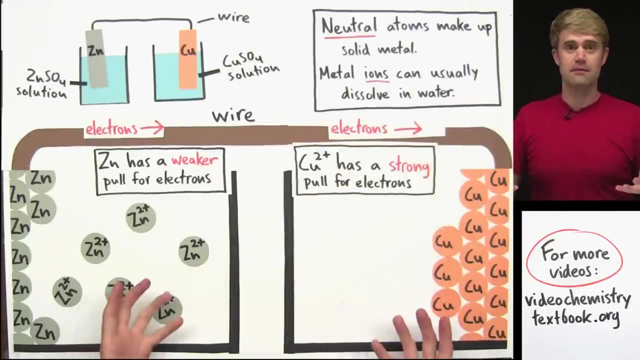 So that is where this electron movement through the wire is coming from. Zinc loses these two electrons. They move through the wire, creating electricity. They come over here and they join up with the Cu2 plus, turning it into neutral copper. We have these electrons moving through the wire here, creating electricity. 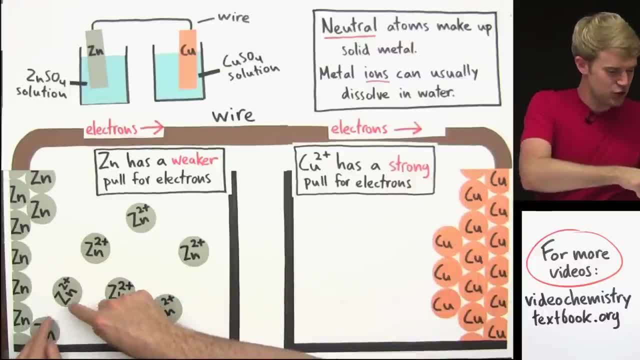 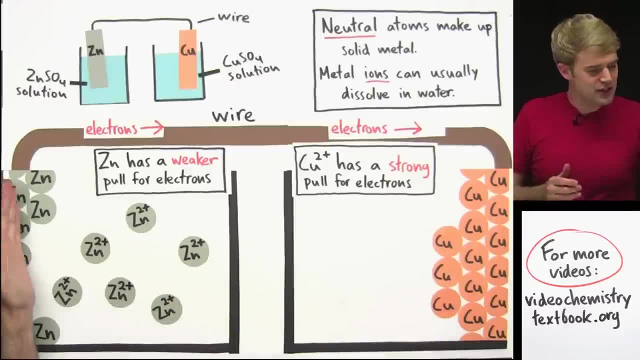 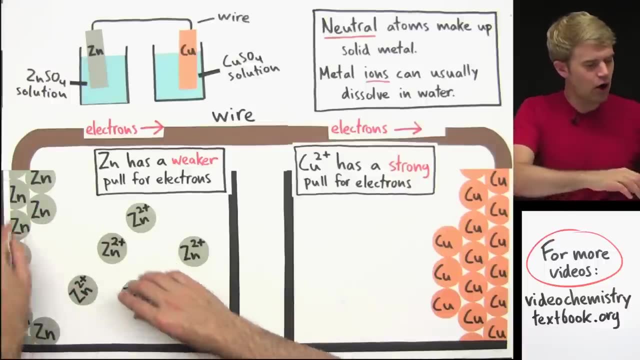 So that is how we get electricity: from these electrons moving from the zinc over here into the copper And if this happens long enough, We actually see these two pieces. These two pieces of metal change, Like these zinc atoms keep coming off of this piece of zinc. 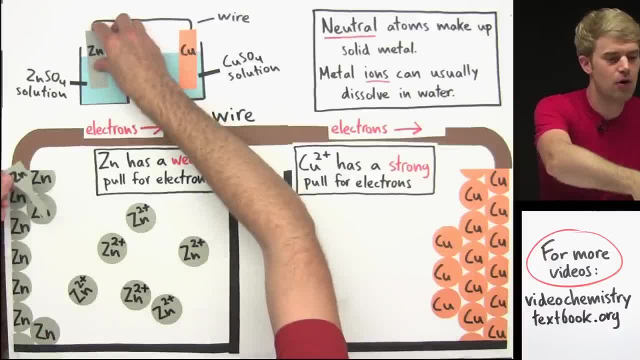 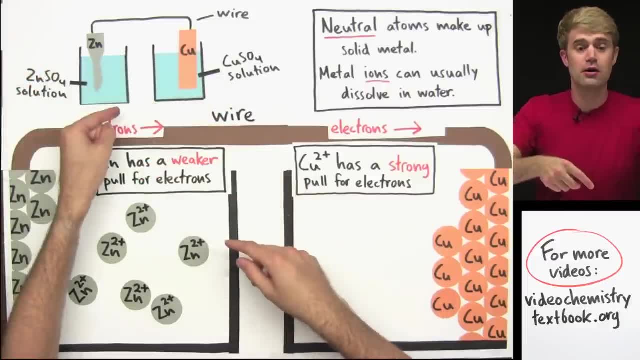 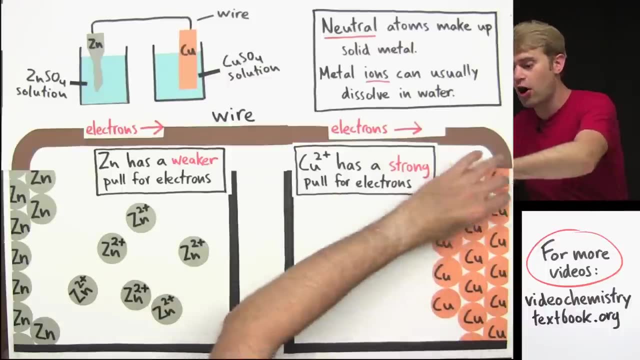 So it is essentially dissolving And over time what we will see is that this piece of zinc actually starts to dissolve. It gets smaller and smaller, But then, on the other hand, those Cu2 plus ions are coming out of solution and are attaching to the solid copper. 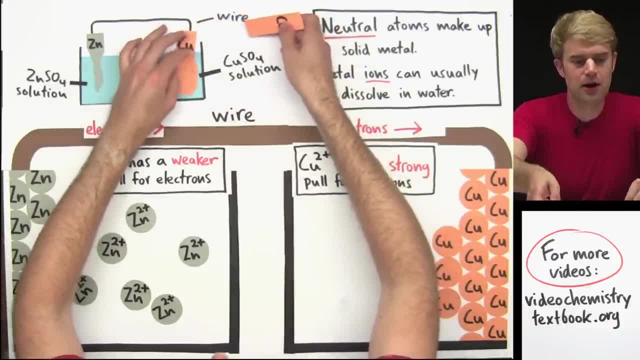 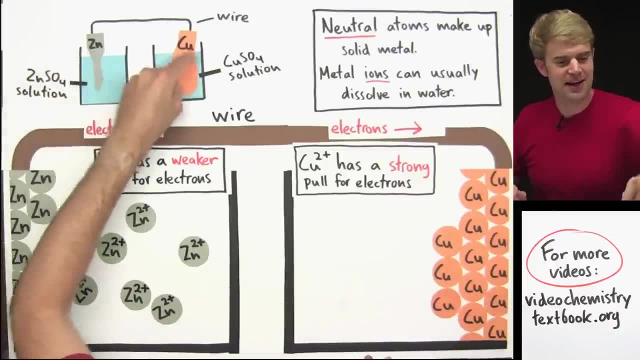 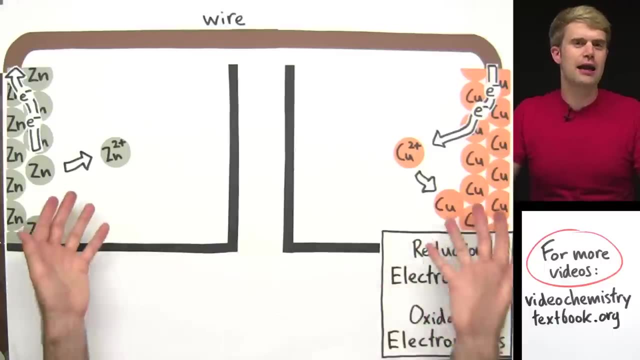 And so They make this piece of solid copper bigger and bigger, And so if we let this voltaic cell run for long enough, we will eventually see that these two pieces of metal actually change size and shape. Here are some diagrams for the process that is happening in the voltaic cell. 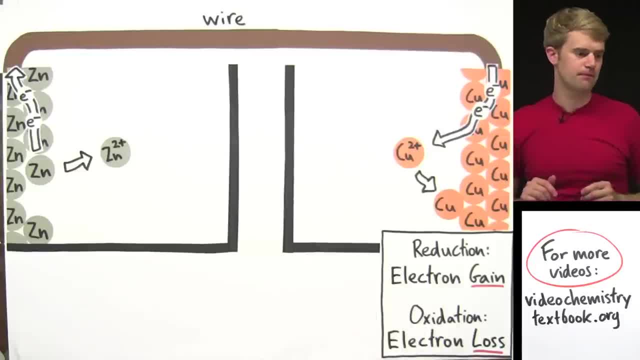 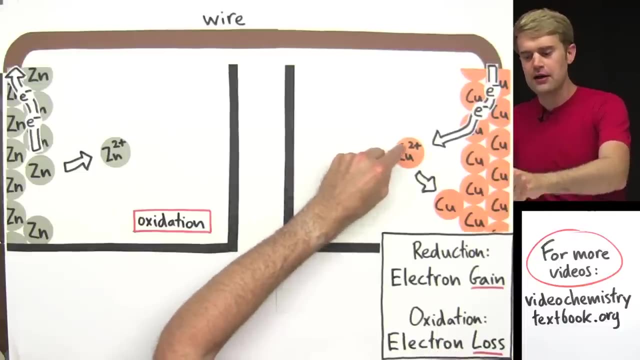 I want to describe what is going on in terms of oxidation and reduction. So over here, One of these neutral zinc atoms is losing oxygen Using electrons. So that means that oxidation is happening on this side of the voltaic cell And over here. 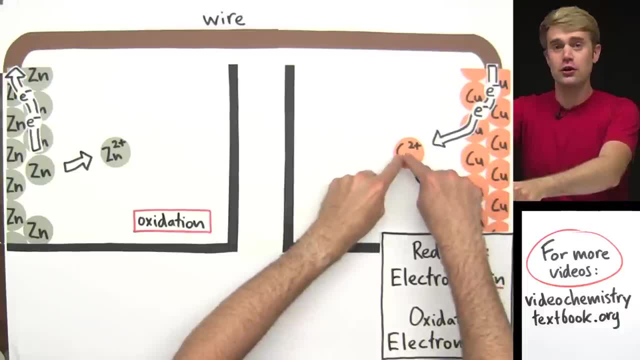 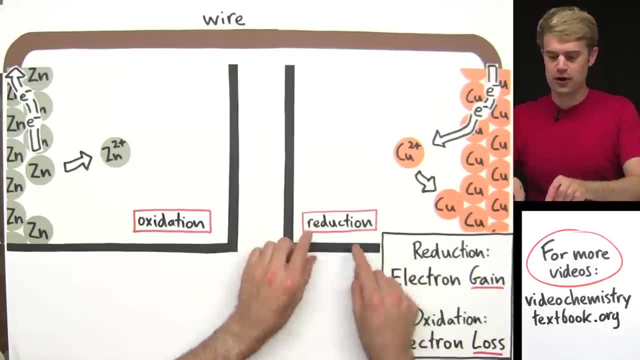 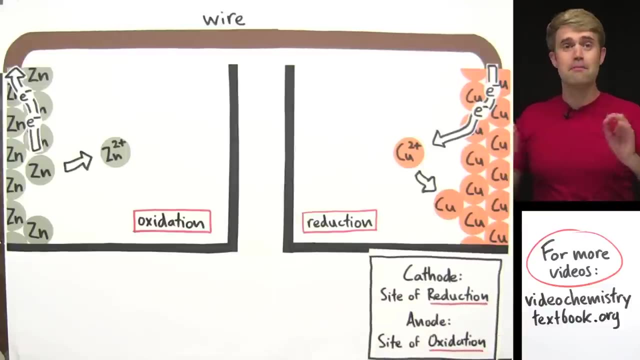 This Cu2 plus ion is gaining two electrons to turn into a neutral copper atom. So reduction or gain of electrons is happening over here. Now we can give names to these two parts of the voltaic cell based on whether oxidation or reduction takes place. 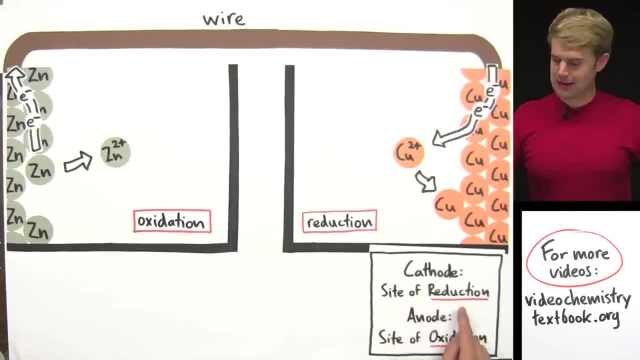 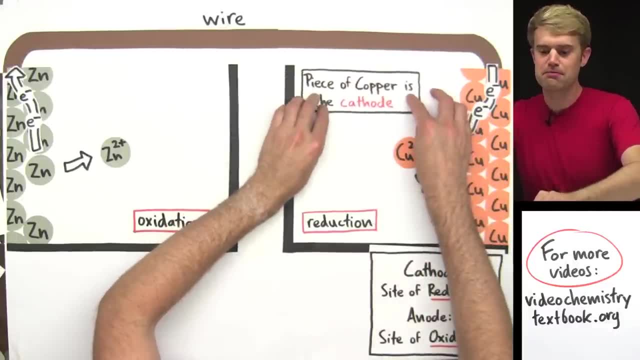 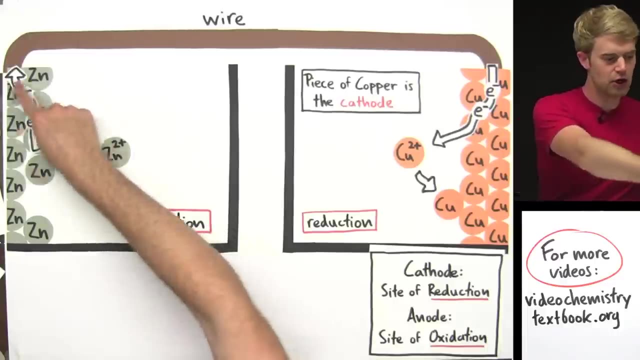 So the cathode is the name that we give for the site of reduction, Where reduction happens. So reduction is happening here, Which means that the piece of copper is the cathode, The site of reduction, And the piece of zinc over here is where oxidation is happening. 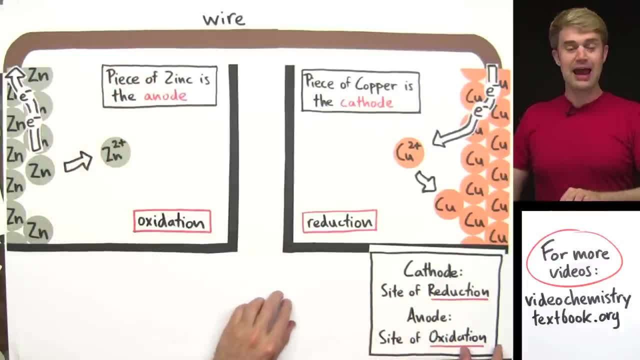 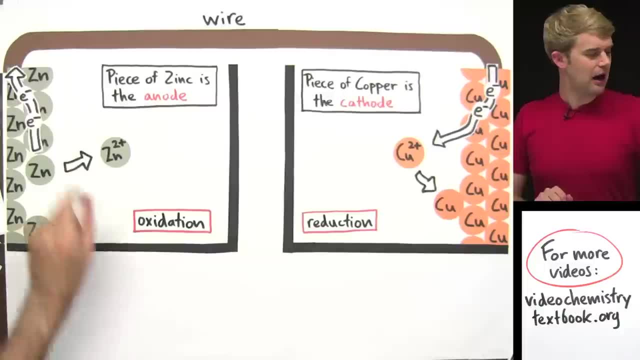 So the piece of zinc is going to be the anode. So reduction at the cathode on copper And oxidation at the anode on zinc. Now let's write reactions for the two processes that are happening here. Okay, First let's write the reaction for reduction. 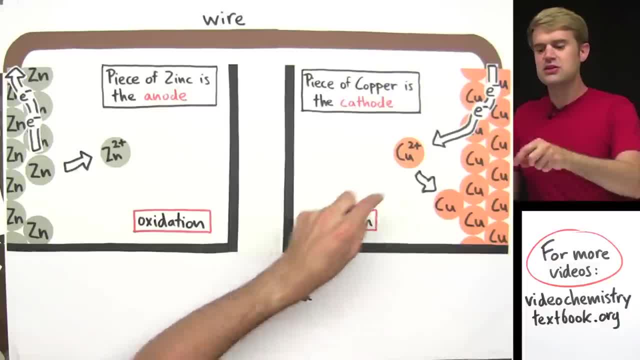 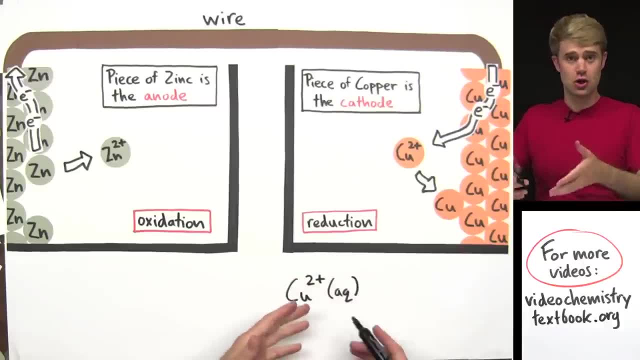 We're starting with Cu2 plus, And this Cu2 plus is dissolved in solution, So I'm going to write that with an aq for aqueous after it, To show that it's dissolved in solution. Now this Cu2 plus Gains. 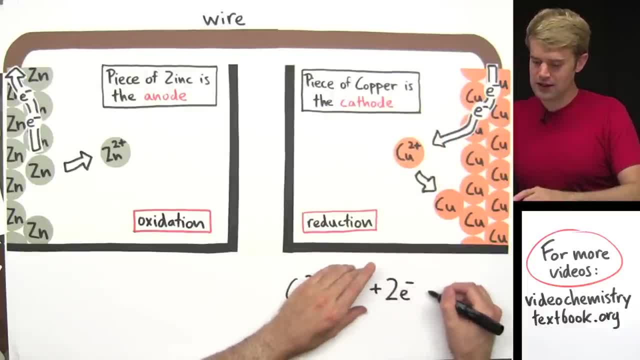 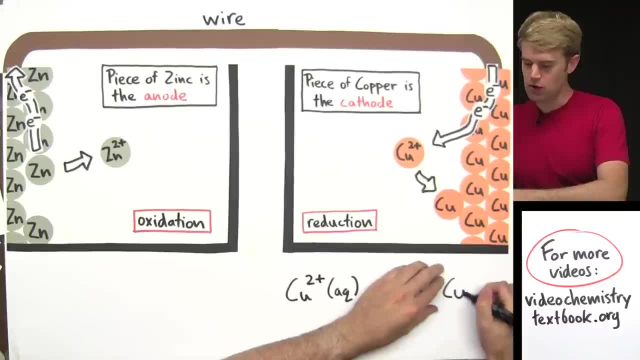 Two electrons, So I'll write plus two e minus, And that gives us a neutral copper atom. So I just write Cu with no charge after it. That shows that it's neutral. And then it's part of the solid metal, So I write an s after it. 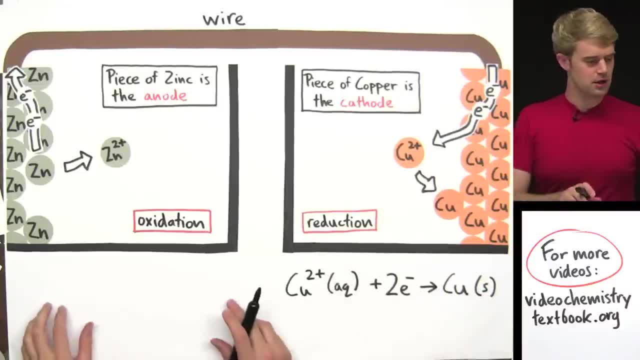 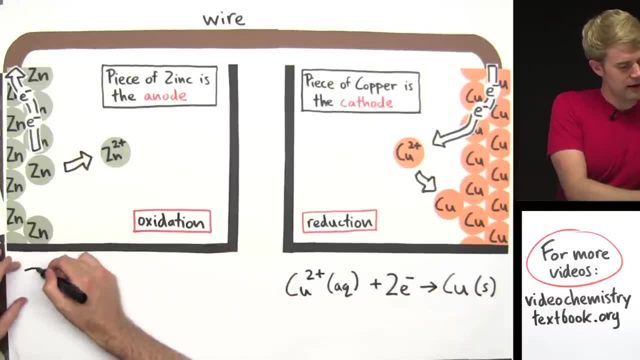 So this is the reaction for the reduction process Over here, The reaction for the oxidation process. We start out with A neutral zinc atom, And this neutral zinc atom is part of the solid piece of zinc. So I'm going to put this s here for solid: 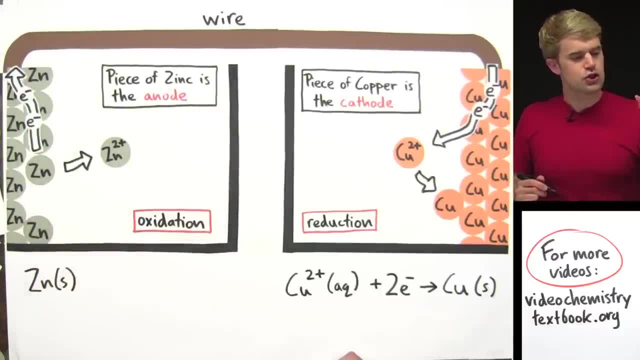 Now it loses two electrons. To show that we lose something in a chemical reaction, we put it on the other side of the arrow. Okay, So I'm not going to write anything right here. I'm going to put this arrow. I'll leave the electrons for last. 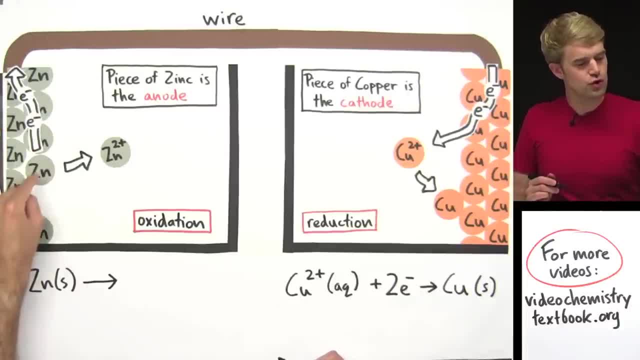 Losing the electrons Turns the neutral zinc atom. I'm going to put the neutral zinc atom into a Zn2 plus ion- Zn2 plus That is now dissolved in solution. So I'll write Aq here And then finally to show that I lost those two electrons here. 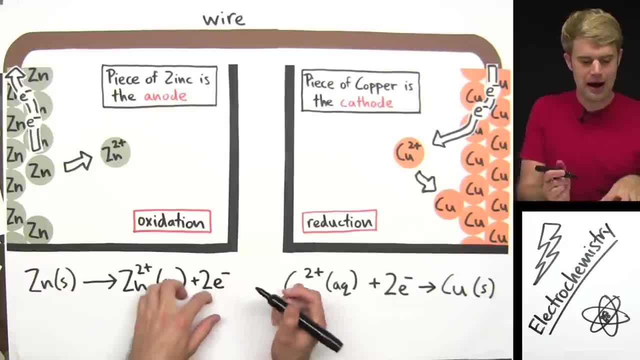 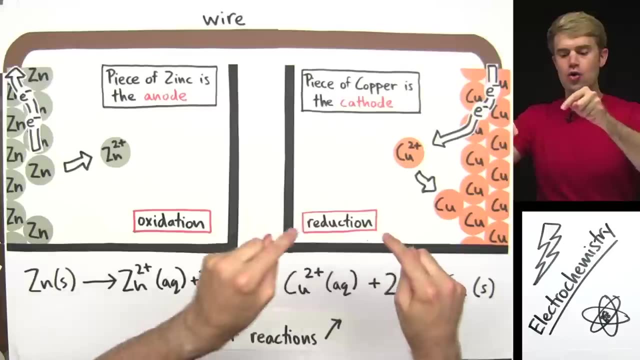 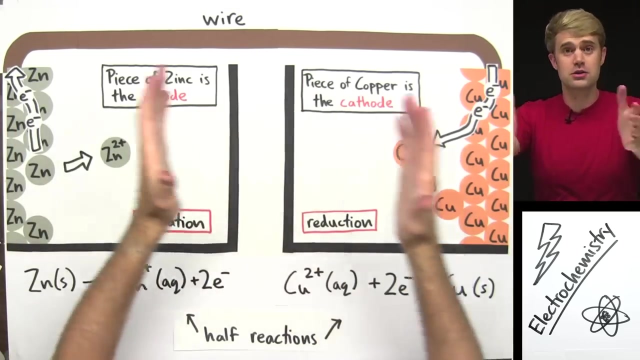 I'll put plus two e minus on this side. So this is the reaction for the oxidation. Now, these two reactions that I wrote, We call them half reactions Because each one of them tells half the story Of the oxidation reduction process. And we can actually give names to these two parts of the voltaic cell, as if each one of 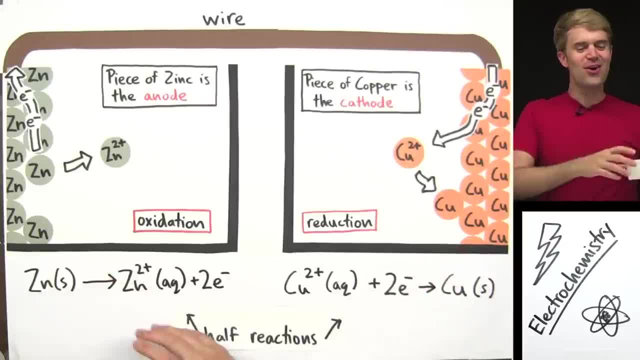 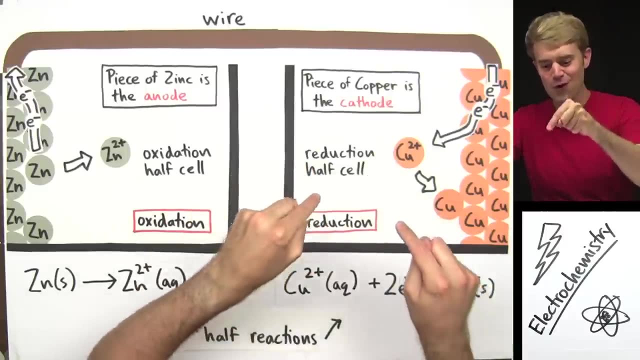 them is half of the big picture. We call this the oxidation half cell. It's half of the voltaic cell where the oxidation is taking place, And we call this the reduction half cell. It's half of the voltaic cell Where reduction is taking place. 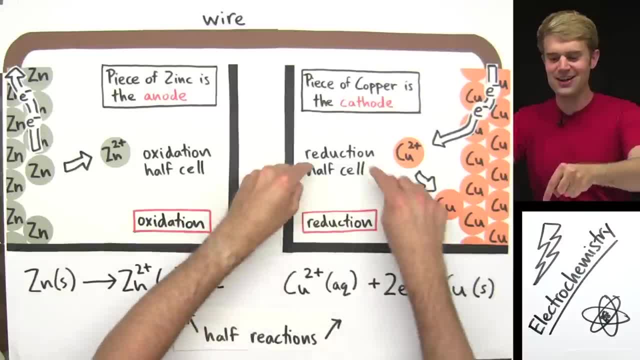 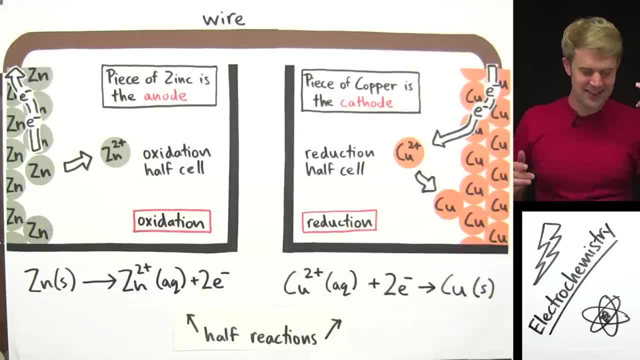 And it is these half reactions that show what's going on in each one of the half shell, In each one of the half cells. I said half shells. It's like Teenage Mutant Ninja Turtles coming back to haunt me from the 80s. 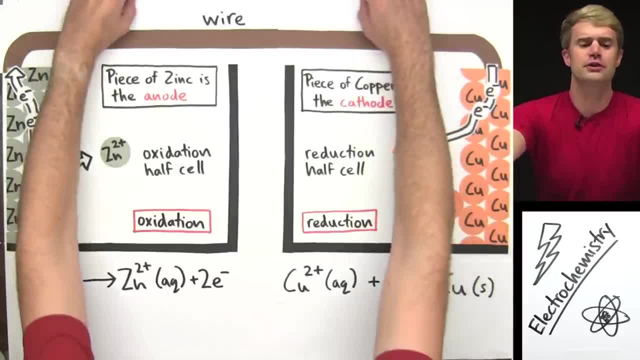 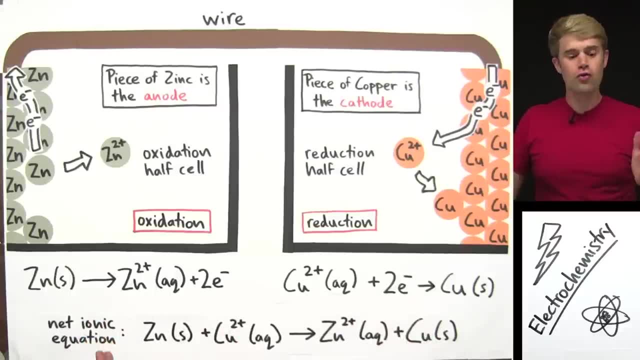 Anyway, we have these two half reactions and we can put them together to get a net ionic equation Which shows the overall oxidation, Oxidation and reduction process. We start with solid neutral zinc and Cu2 plus ion And then at the end of the process we're left with zinc 2 plus ion and then we have solid. 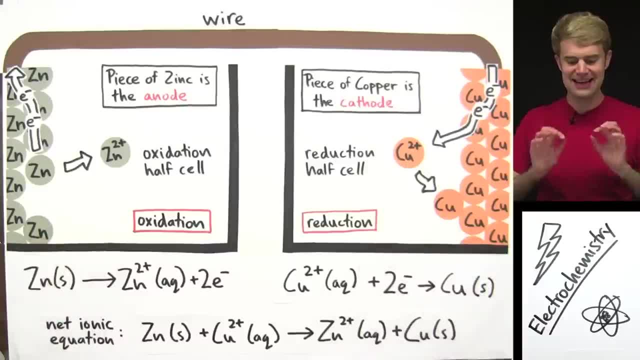 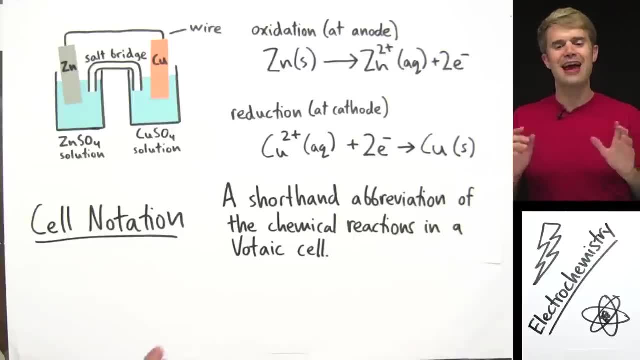 copper. This is the net ionic equation that we get from adding together these two half reactions. Now, when we're talking about voltaic cells, we're often asked to represent them in cell notation, Which is a shorthand abbreviation of the chemical reactions in the voltaic cell. 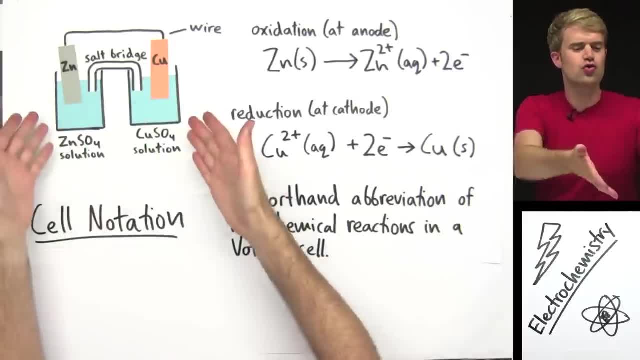 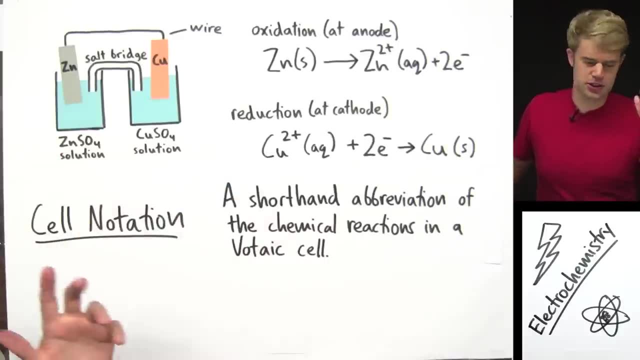 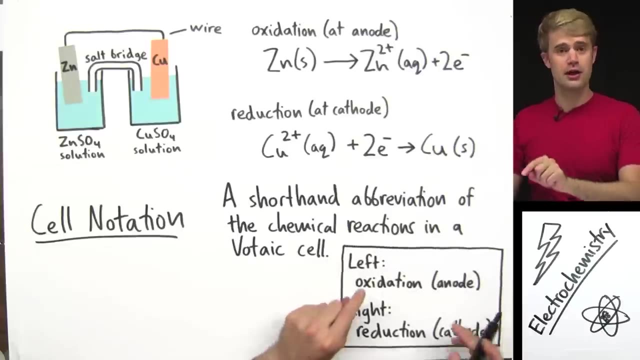 It's a way that we can show what's going on without drawing a picture of the whole thing. Cell notation is sometimes referred to as a cell diagram, just so you know. So here's how we would write what's going on in this voltaic cell, using cell notation. 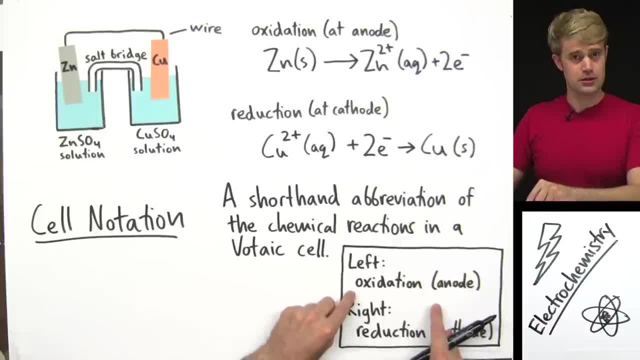 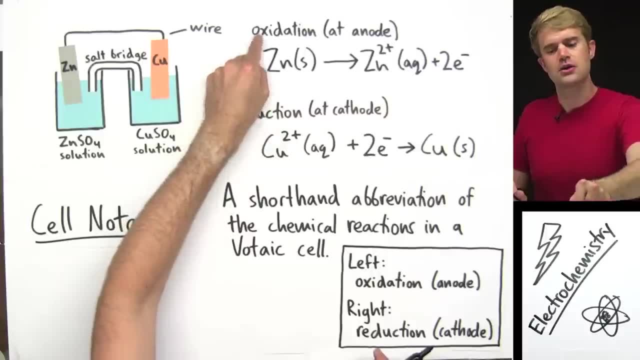 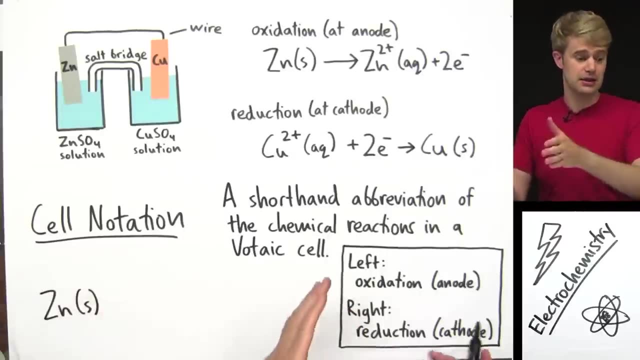 We start on the left with the oxidation process. Okay, How does the oxidation process start? Well, I have the half reaction up here. It starts with solid zinc, So I will write Zn solid right here. That's how the oxidation begins. 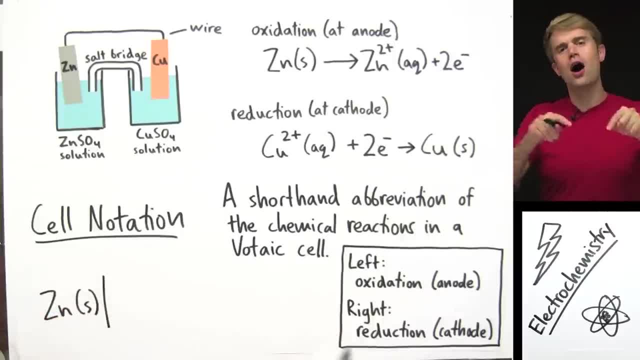 Then I put this line here and I show what we end up with in the oxidation process, which is Zn2 plus. So Zn2 plus and that is dissolved in water. It's part of the solution. It's aqueous, Okay. 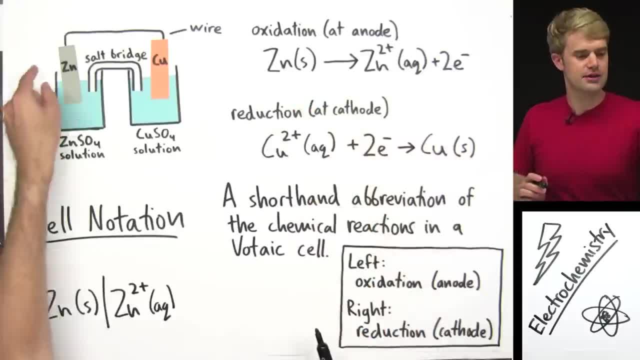 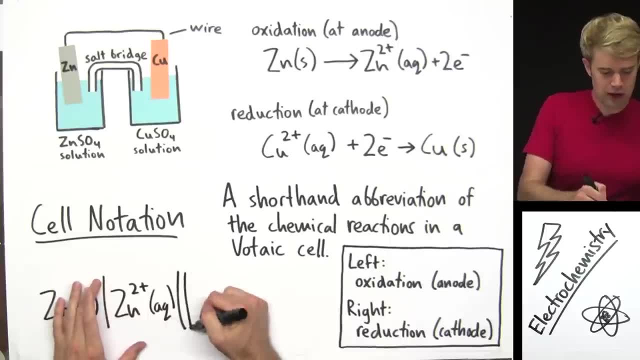 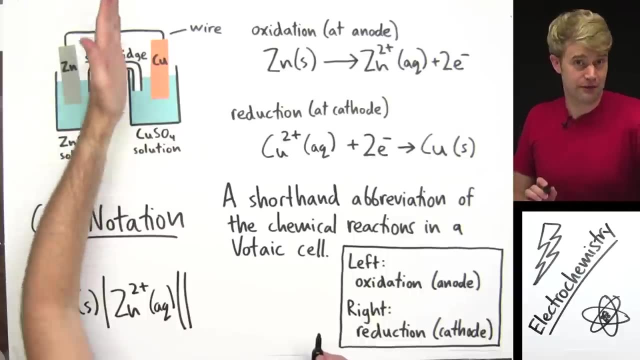 So this shows the oxidation process that happens in the half cell over here. Okay, Then I put two lines like this: and these two lines represent the physical boundary between these two half cells, or you can think of them representing the salt bridge. Okay, Now, on the right, I put information about the reduction process. 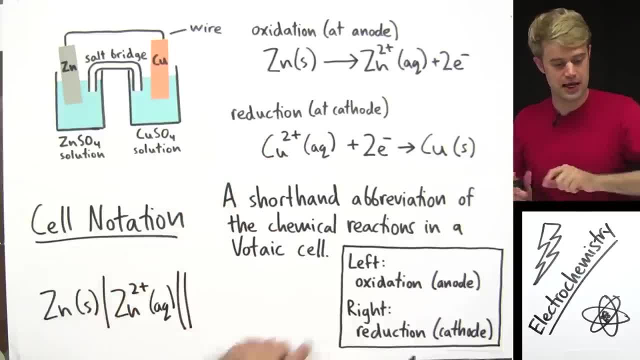 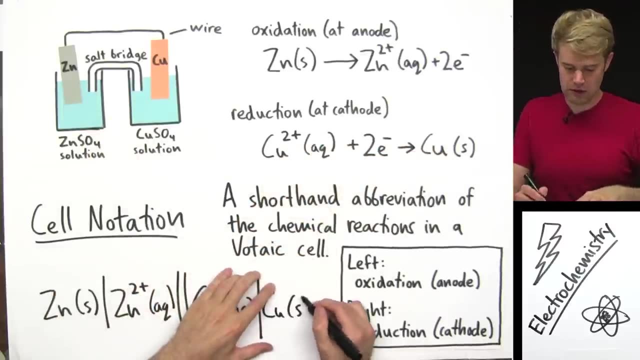 So the reduction process begins with C2.. C2 plus aqueous, C2 plus aqueous, and then I will put another one of these lines and the reduction process ends with Cu solid. So there's Cu solid. So this is how we can sum up what's going on in this voltaic cell, using cell notation. 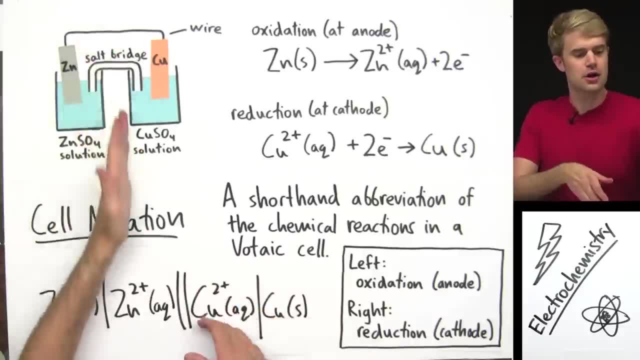 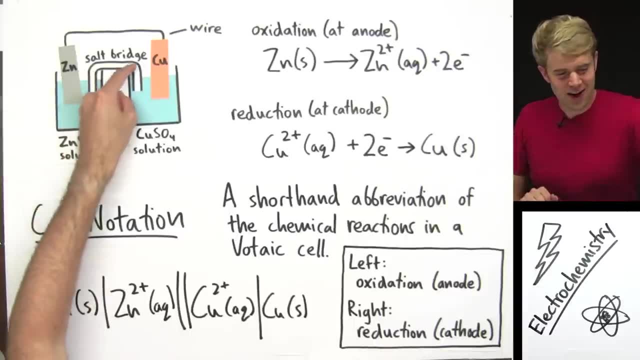 We have the oxidation process and then two lines showing the boundary and then we have the reduction process. So, finally, we've talked a little bit about the salt bridge and I said we'd discuss it at the very end. So let me take a minute or two and explain what the salt bridge is, what it does, and 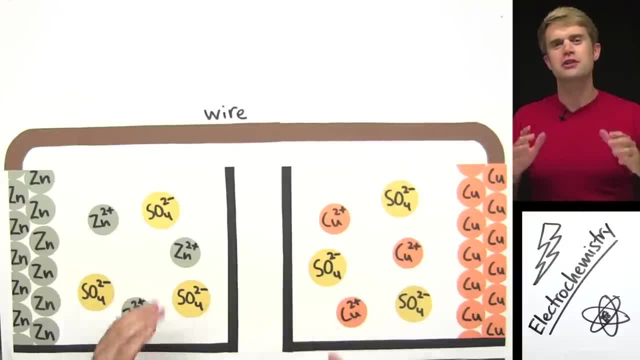 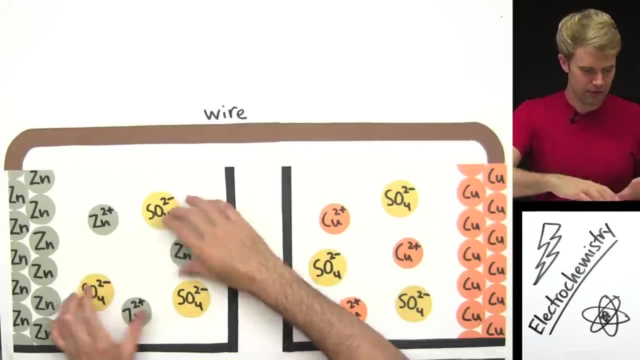 why it's important in a voltaic cell. The salt bridge helps to balance out charge in the voltaic cell. Here's what I mean. The two solutions are made up of both positive ions and negative ions. I didn't know that I didn't show the negative ions before. 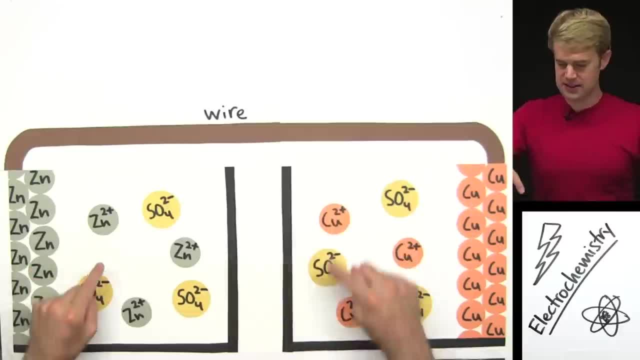 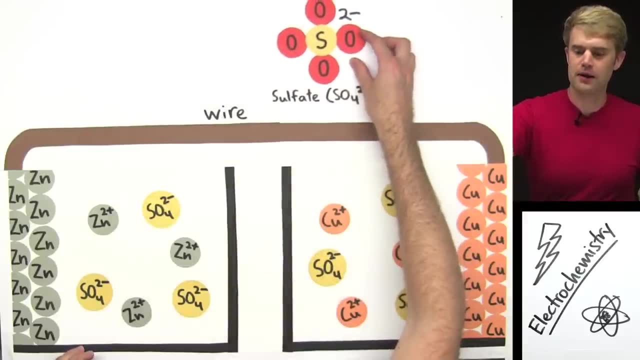 Those are these yellow things. I just showed the zinc and the copper. But along with these metal ions are these polyatomic ions, sulfate SO4, 2 minus. It's a sulfur with four oxygens and the whole thing has a 2 minus charge. 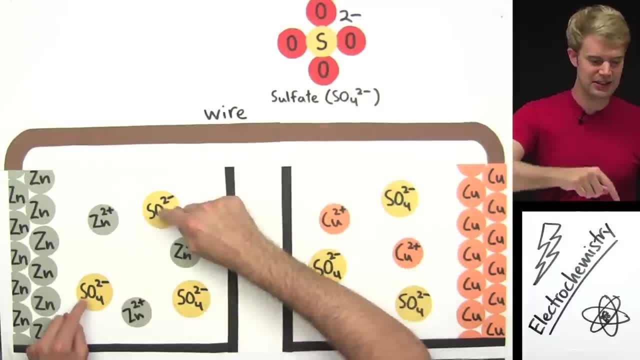 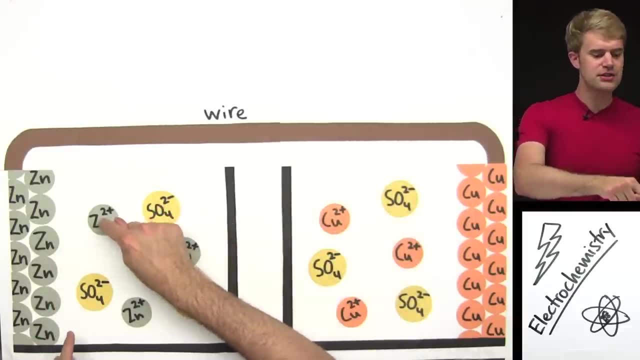 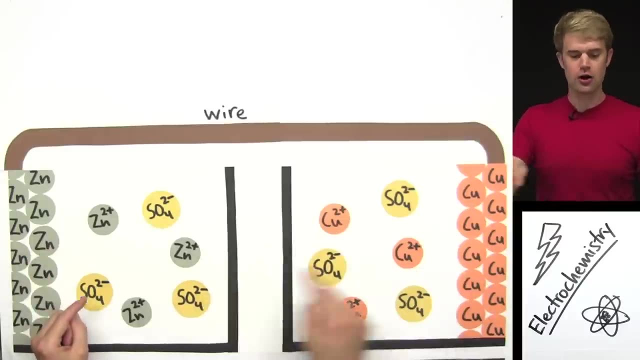 I didn't want to have to keep using this thing, so I've just abbreviated these as SO4 2 minus. But the point is The negative charge from the sulfate balances out the positive charge from the zinc or from the copper. So right here in my two half cells the charges are balanced out. 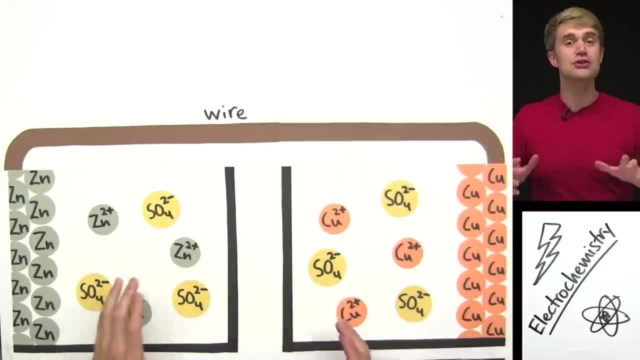 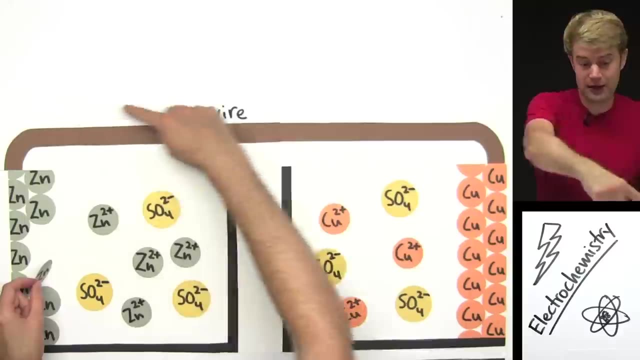 But let's look at what happens as the voltaic cell begins to run for a while Over here. these zinc atoms are going to give electrons to copper, so they are going to end up with a charge. I'm not showing the electrons here, Okay. 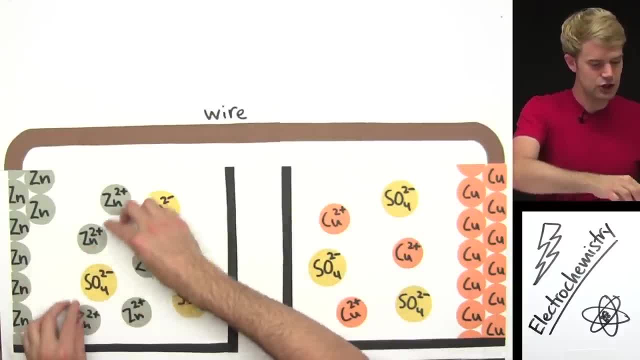 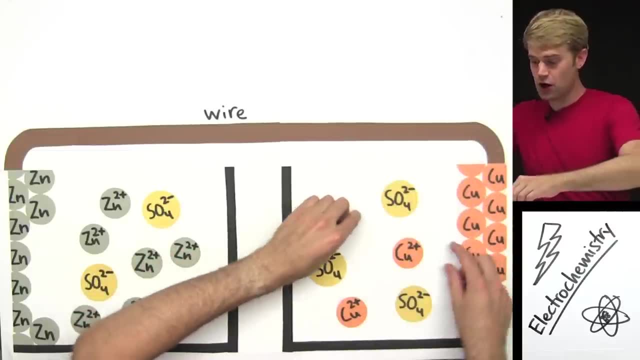 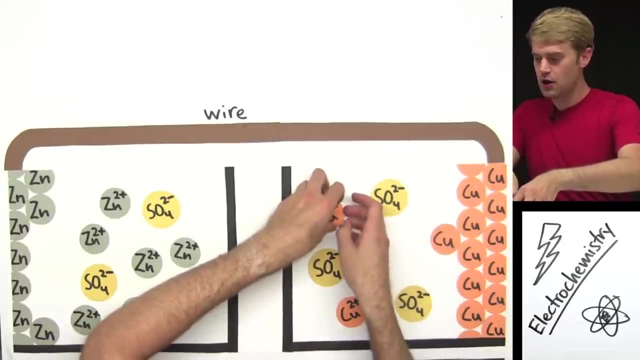 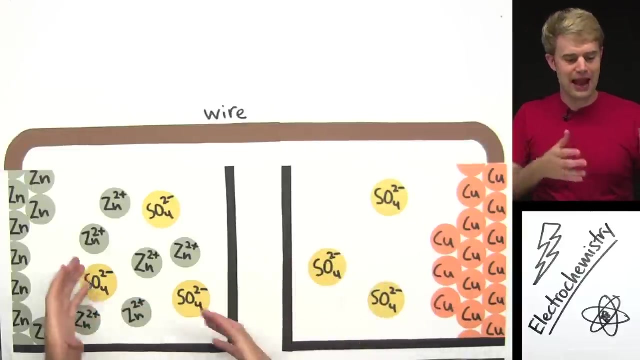 This is something sent up here. as these turn into Zn2 plus ions and as they enter the solution Now over here, as electrons come over, these Cu2 plus ions will turn into neutrally charged copper atoms and attach to the metal. Now look at what's happened to the charge here. 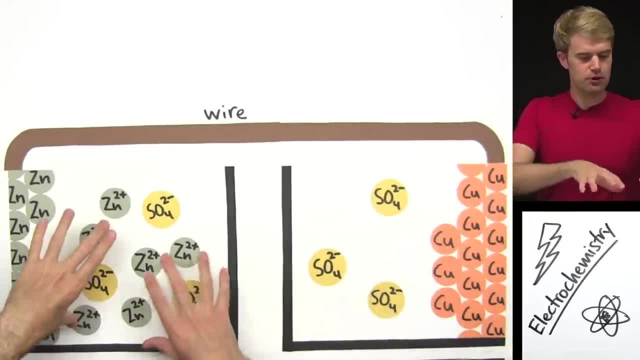 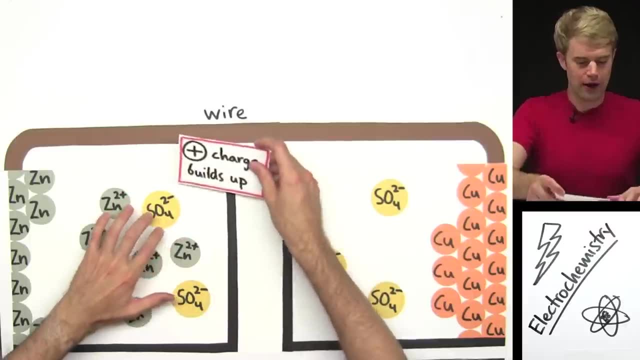 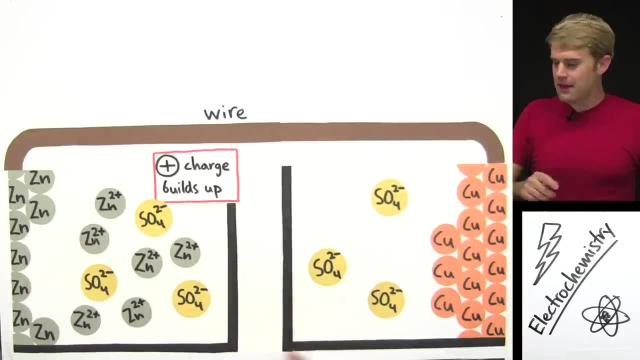 Okay, Now we have all of these Zn2 plus ions, We have Zn2 pluses, but we have only a few of the SO4 2 minuses. So after just a little while positive charge really begins to build up in this half cell. 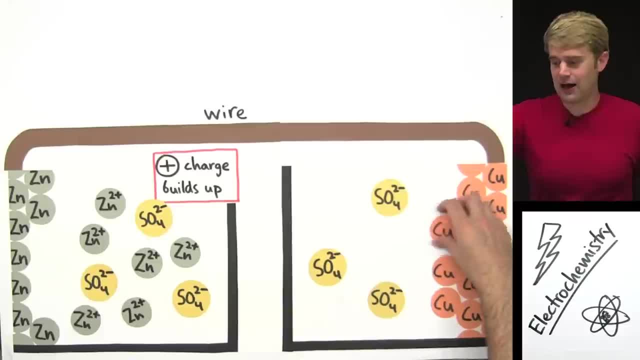 And then over here as the positively charged ions like this lose their charge by gaining electrons and turn into neutrally charged copper. Now there are a whole lot more SO4 2 minuses than there are Cu2 pluses, So a negative charge begins to build up on this side. 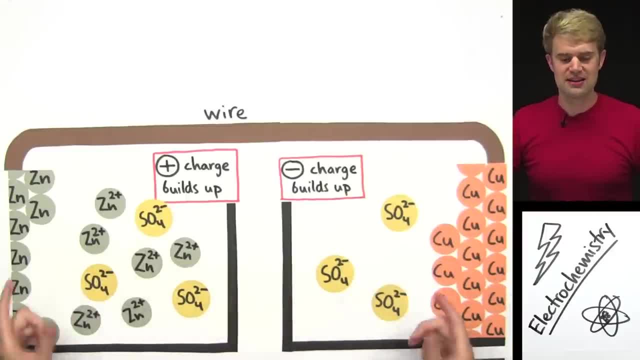 And if this positive and negative charge build up too much, the cell can't run anymore, It can't continue to make electricity. So that is where the salt bridge comes in. Let me get rid of this wire and show you what the salt bridge looks like. 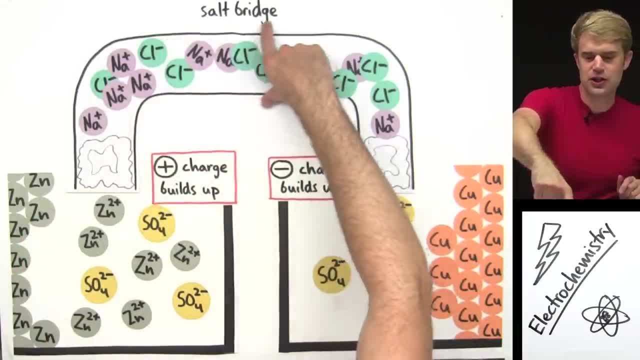 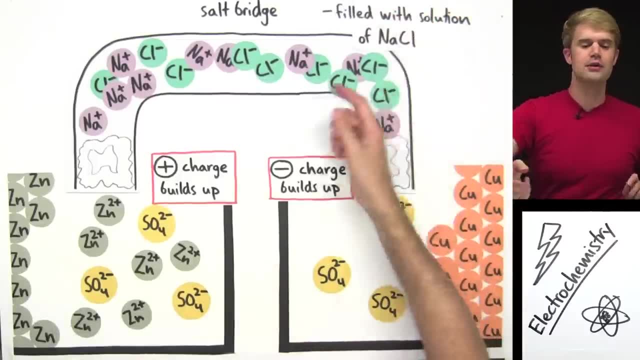 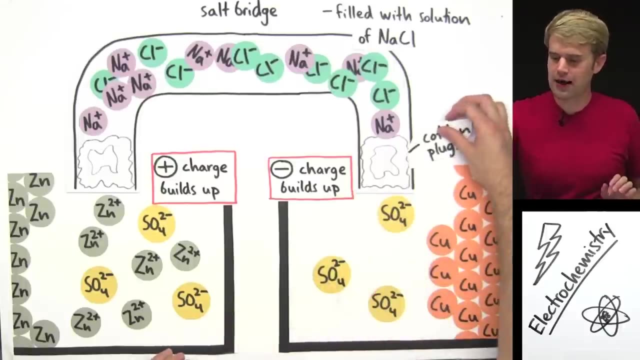 Here is the salt bridge. It is a tube Shaped like an upside down U that, in our case, is filled with sodium chloride And you can see the Na plus and the Cl minus ions. Now, at the ends of the salt bridge there are cotton plugs. a little bit of cotton there. 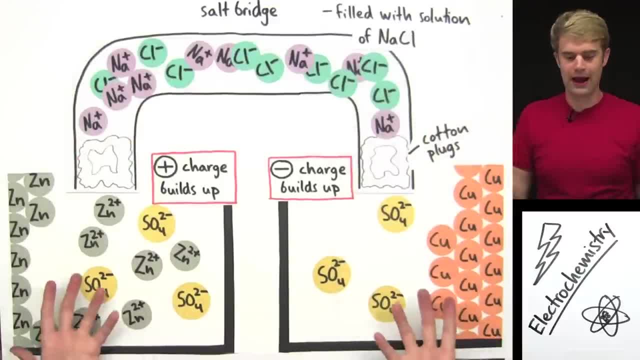 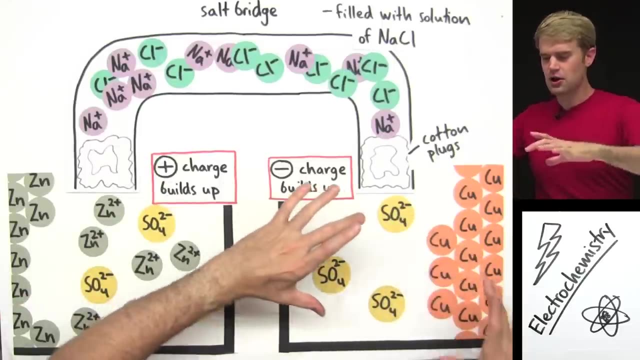 And the cotton prevents the solution from just pouring out into the half cells. But these ions are able to slowly pass through the cotton plugs And here is what happens. We said that negative charge is going to start building up in the half cell over here. 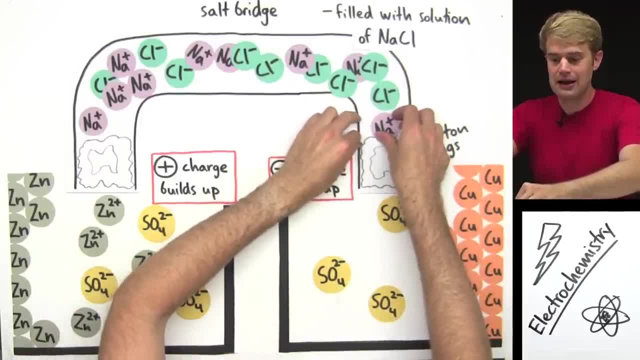 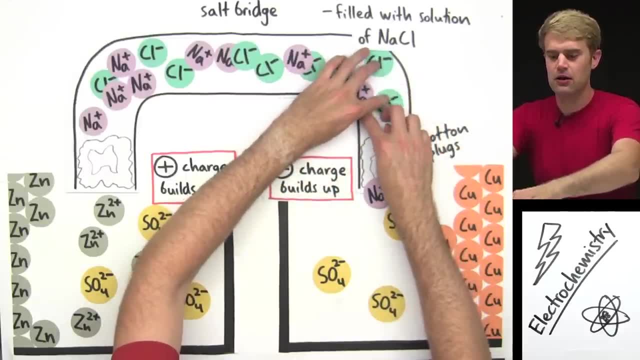 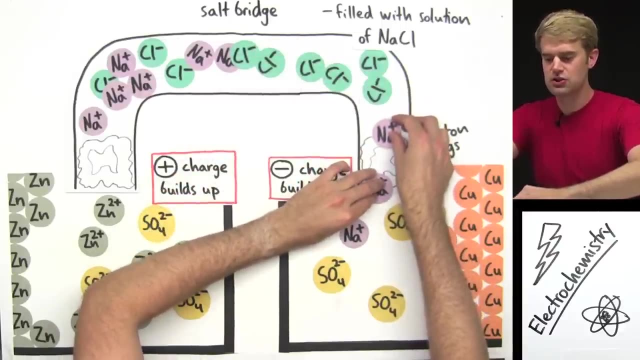 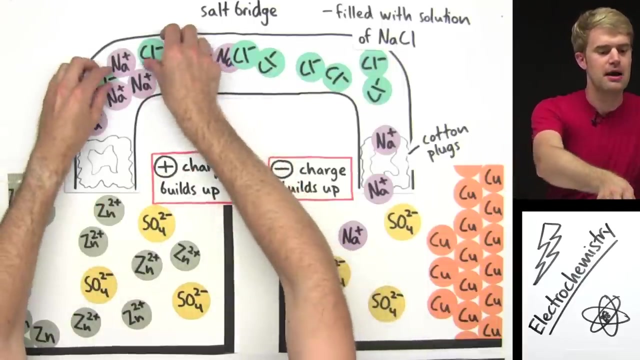 And so the positively charged Na Na plus is going to begin moving over into this half cell to help balance out the charge. So the Na plus ions are going to begin moving in this direction to balance out the negative charge. And over here we said that positive charge begins to build up. 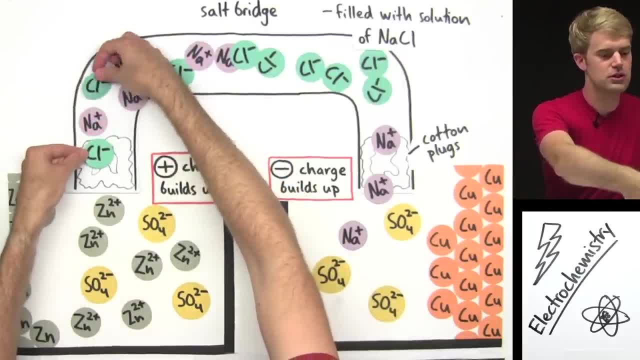 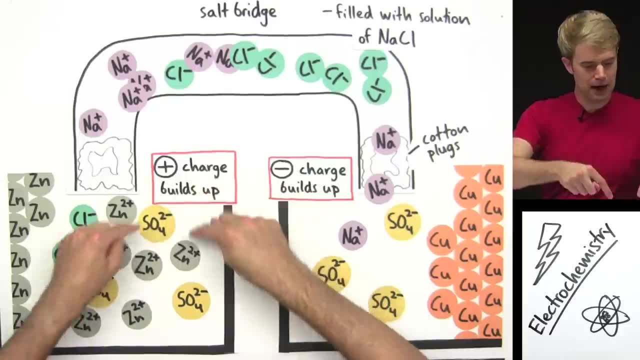 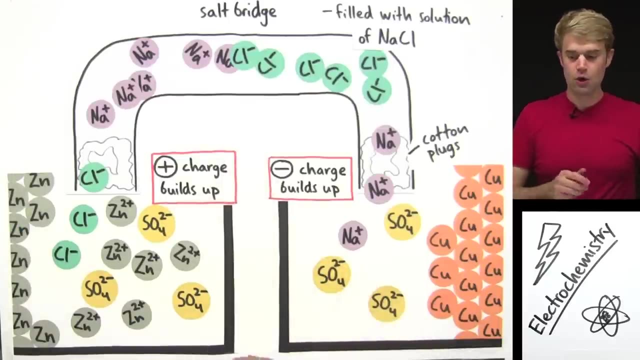 The Cl minus ions are going to begin moving through the salt bridge to come out through the cotton and help to balance out the positive charge that builds up on this side of the voltaic cell. So over time, what we are going to see is we are going to see that the Cl minuses move. 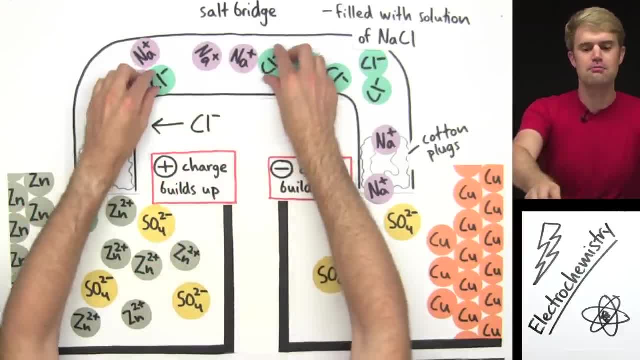 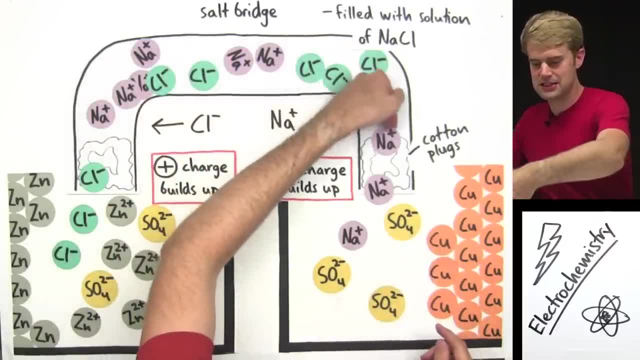 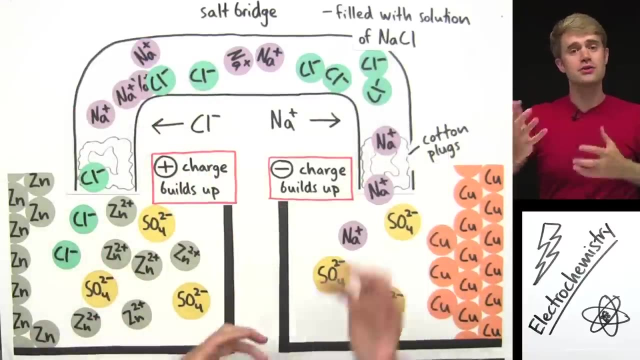 in this direction to balance out the positive charge, And then we will see that the Na pluses begin to move to this side to balance out the negative charge that builds up. here A salt bridge helps to balance these charges, to make sure that they don't build up too. 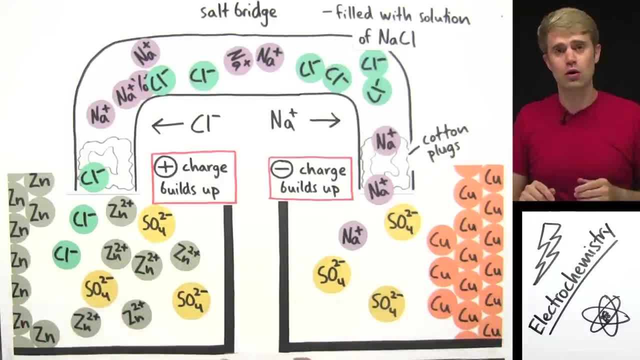 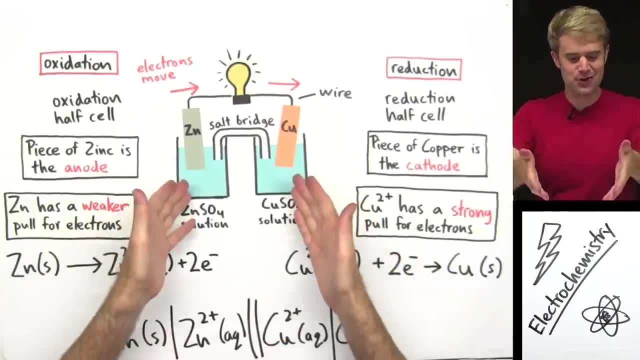 much, and that would prevent the voltaic cell from being able to work. Wow, so we just learned so much about galvanic or voltaic cells. Okay, So here is the basic structure. I am going to show you the basic structure. So here is the basic structure of a voltaic cell. 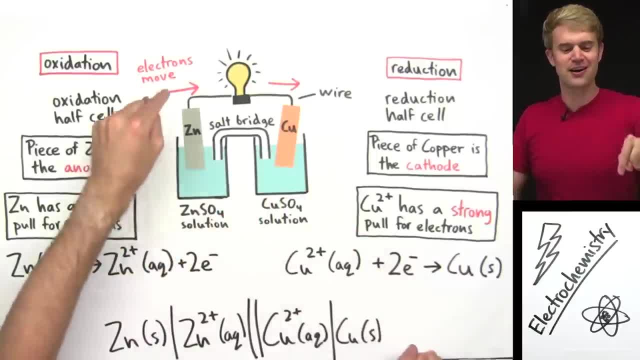 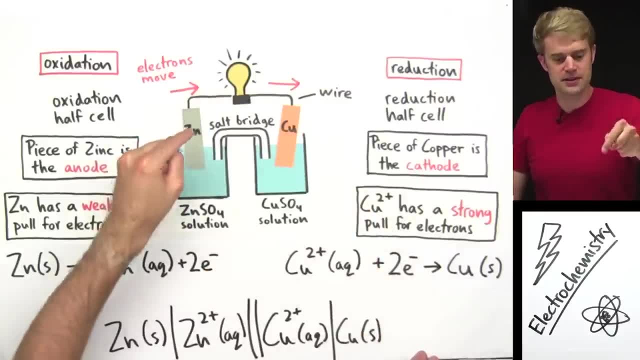 We have the zinc sulfate solution here, copper sulfate solution here we have zinc metal and copper metal. Now, when we hook this all together, electrons start flowing from the zinc to the copper, and that is because copper- that is in the solution- has a strong pull for electrons, whereas 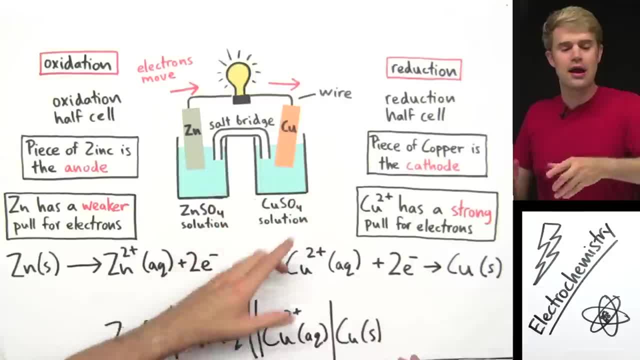 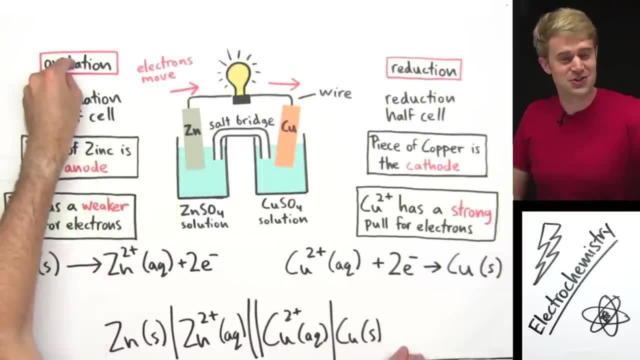 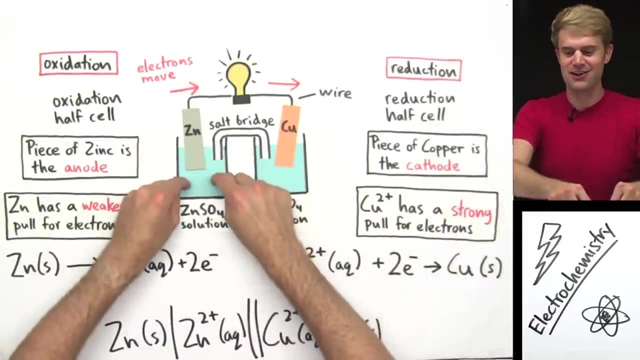 the zinc has a weaker pull, so the copper wins. As electrons move from the zinc to the copper, they are lost in the zinc, so oxidation takes place, So electrons are gained here in the copper, so reduction takes place over here. We call this the oxidation half cell and we call this the reduction half cell because 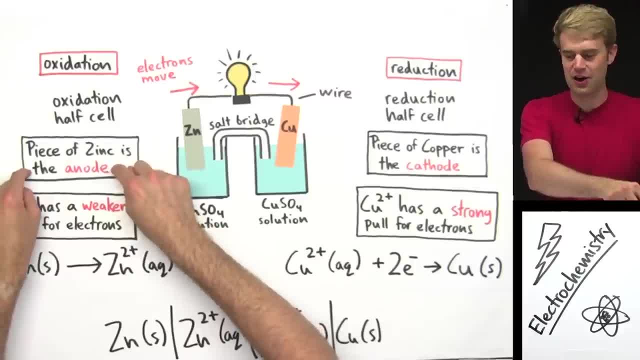 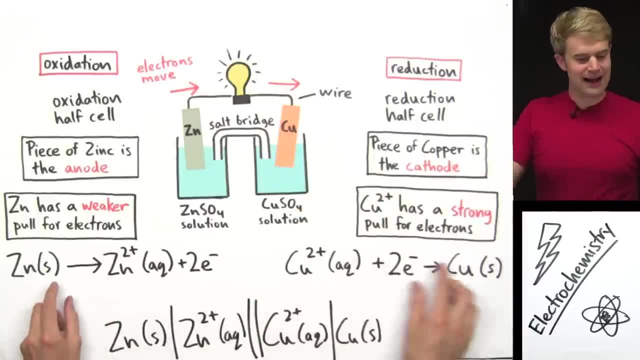 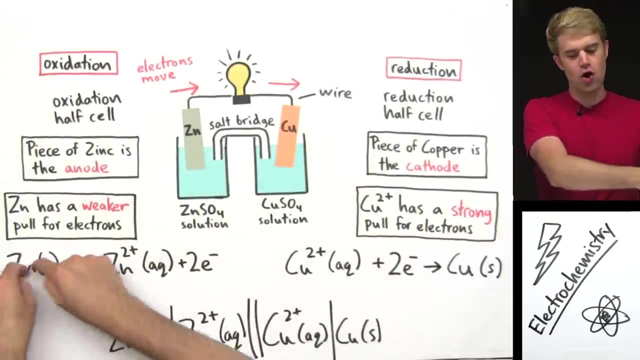 oxidation is happening over here. The piece of zinc is the anode, because reduction is happening over here. The piece of copper is the cathode. Then, finally, we can write half reactions for the two processes that are happening in the different half cells. Here is solid zinc losing two electrons because they are moving out.